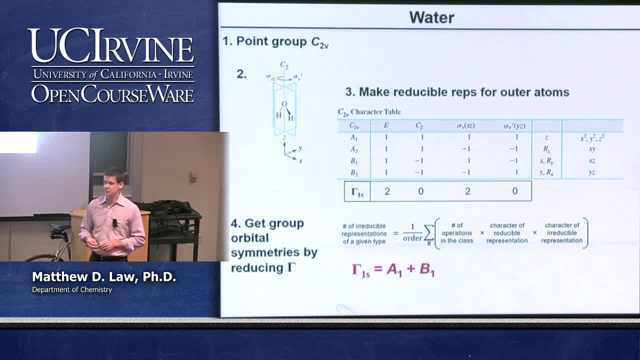 So in water, all we have to do to understand the molecular-orbital diagram is to look at the group orbitals, which are formed from the 1s orbitals of hydrogens, and try to pair those with the center atom orbitals, the 2s and the 2p orbitals of oxygen. 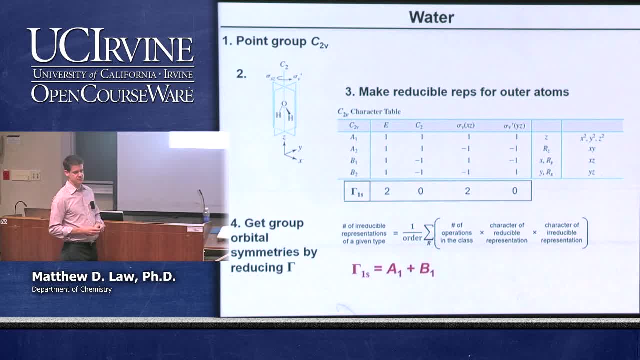 What we want to do, then, to get the group orbitals is to describe, to build a reducible representation for the 1s orbitals, for the two 1s orbitals, And that reducible representation is shown here for the four different symmetry classes, operation classes. 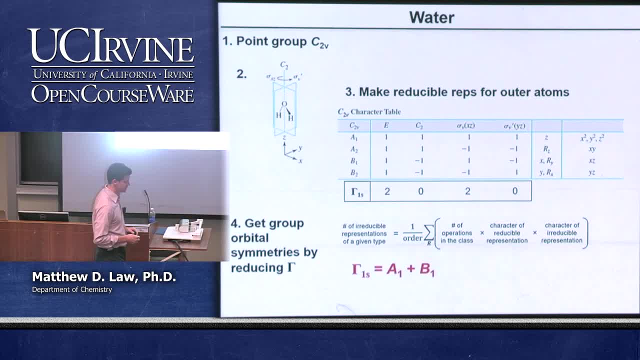 We can take this reducible representation and we can reduce it using our normal equation and that gets us: the reducible representation for the 1s orbitals is equal to a1 plus b1.. So those are the two irreducible representations that go into the reducible. 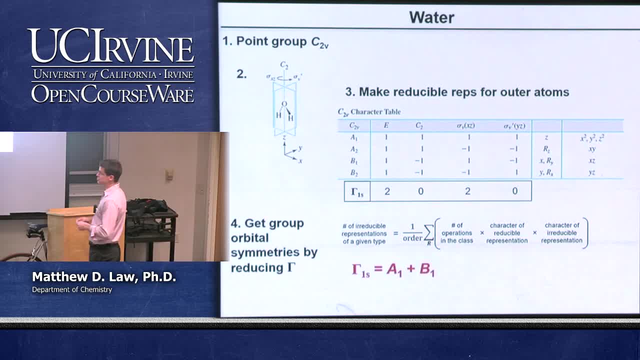 And so we expect then, the symmetry of the two group orbitals that we build from the 1s's to be a1 and b1 symmetry. And remember, because we're only dealing with two group orbitals, there's really only two ways that we can build the group orbital up. 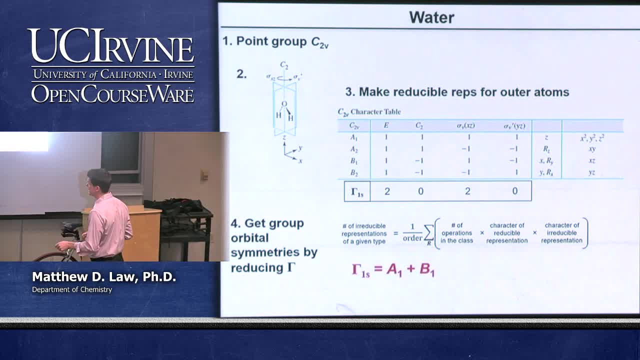 We can take the sum or we can take the difference, And so this one's going to be the sum and this one's going to be the difference. We can tell that right away, because this is the totally symmetric representation in this point group. 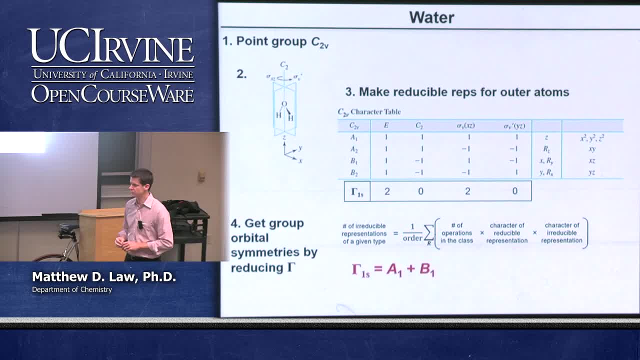 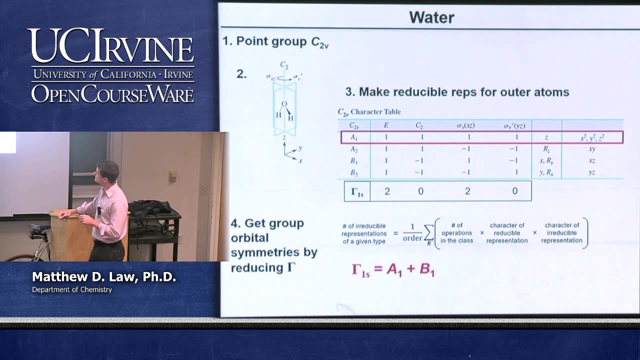 And so it has to be the totally equivalent representation. Okay, what else can we tell just reading off the character table? Well, we want to understand how these two group orbitals from the hydrogens are going to interact with the oxygen. And we can read that right off the table, because a1 has the same symmetry as the z axis. 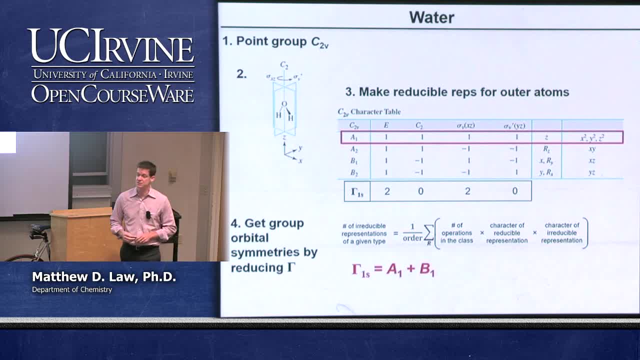 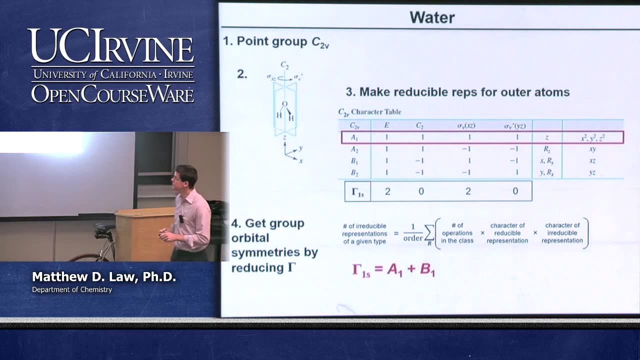 So we expect the pz orbital on oxygen to interact, because it's going to have the same symmetry As the a1 group orbital. Also, the s orbital on oxygen is going to have completely symmetric representation, as it always does. Okay, so s and pz should interact with a1.. 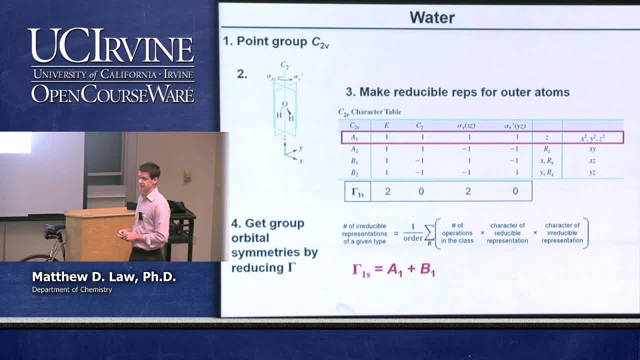 What about b1?? Well, we look over on b1 and it has the same symmetry as x, So the px orbital on oxygen should interact with the b1.. What about the py orbital? Well, it doesn't have a symmetry matched pair in the group orbitals. 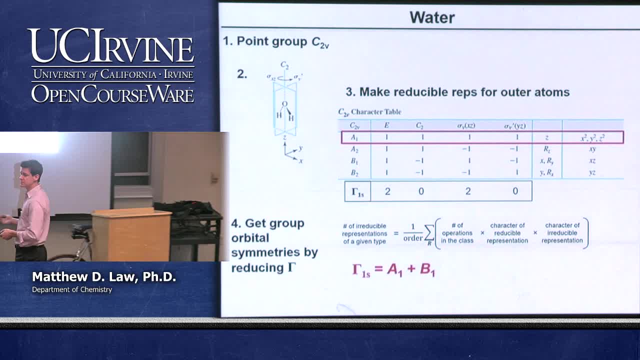 So we expect? The prediction is that the py is going to be totally neutral. It's going to be non-bonding because it has no symmetry pair, And my clicker has just died somehow, Or my computer froze, which would be even better. 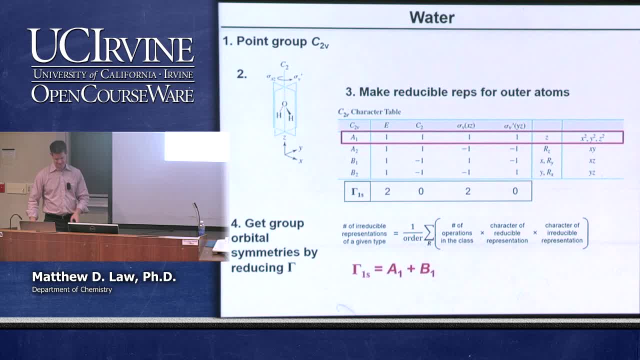 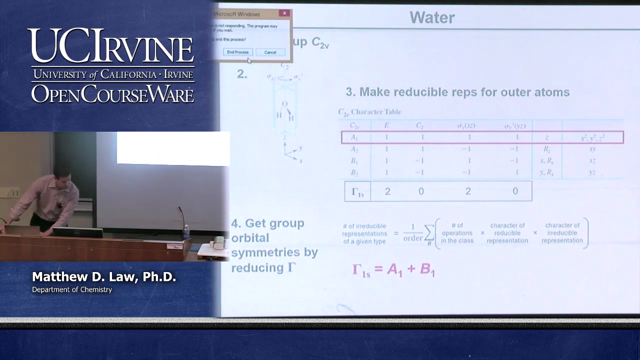 Yeah, and it's the latter? All right, Let's see what we can do about this quickly. And then there's the blue circle of fun. This is such a bizarre problem because nine times out of ten there's no issue. Every once in a while. 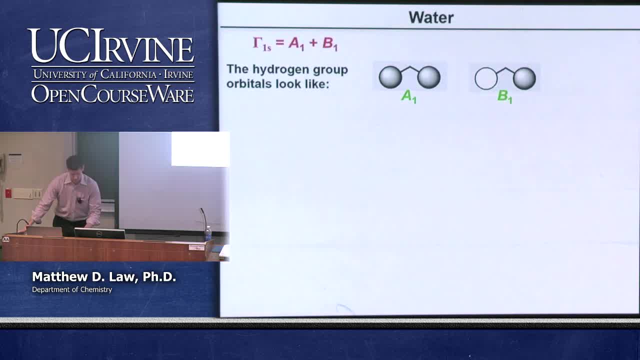 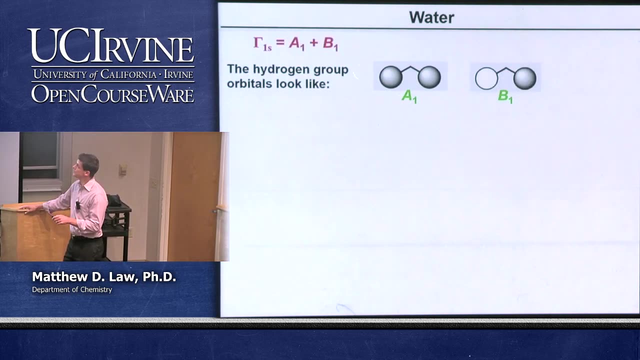 Okay, All right, Let's see if that does it. All right, The electrons were crossed there momentarily, Okay, So what we do- We went through all this, And then what we do is we look at how the actual, You know, in our case, the shading diagram of these two orbitals is going to look. 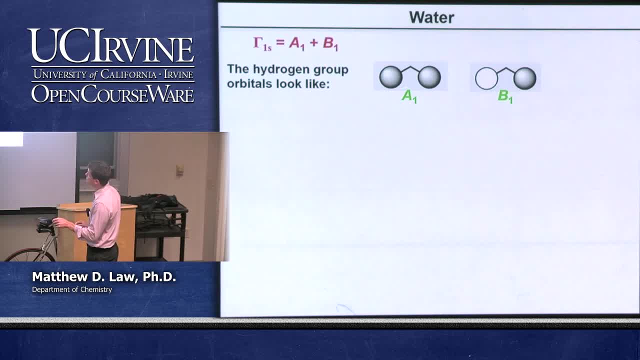 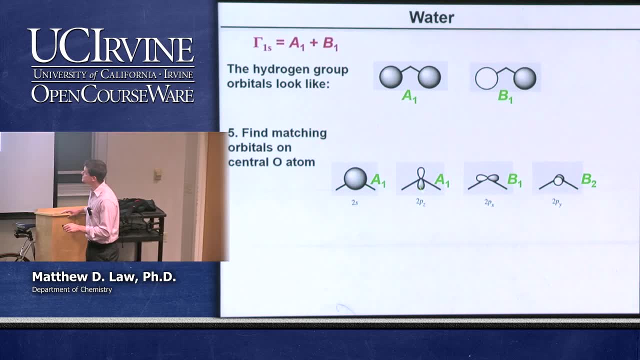 The a1 is totally symmetric, So we just take the two 1s orbitals of the same sign. What do the orbitals look like on oxygen? Well, we said the s orbital is a1, as it must be. The pz orbital is also a1.. 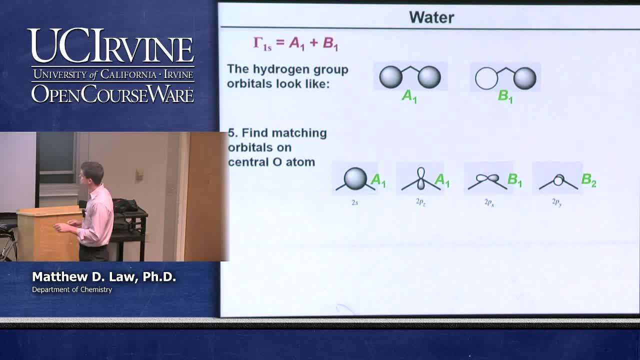 So it has the same characters for the different symmetry operations. Here's the b1 that's going to match with this b1.. So this is the 2px, And then the 2py has totally different symmetry, Right, And so you can see right away that the 2py 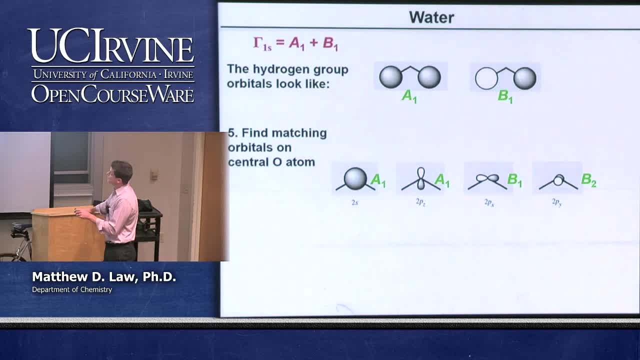 Because it's coming out at you in this picture- Has zero overlap by symmetry with this orbital And it has zero overlap by symmetry with that orbital And that's why we can tell and confirm that this one is going to be non-bonding. 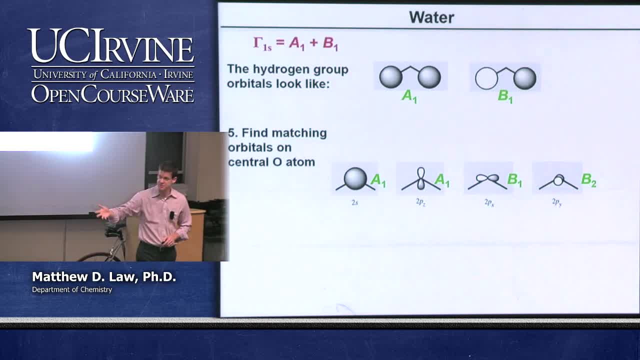 We have six total orbitals that we need to worry about. So we're going to have six MOs, as we always have. You know, equal number of MOs to AOs. We have these interactions, We have these interactions And this is the odd guy out. 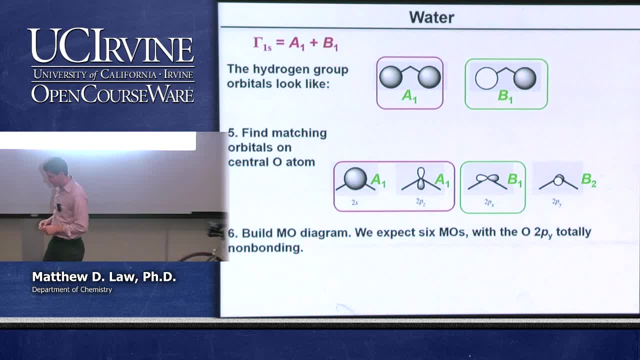 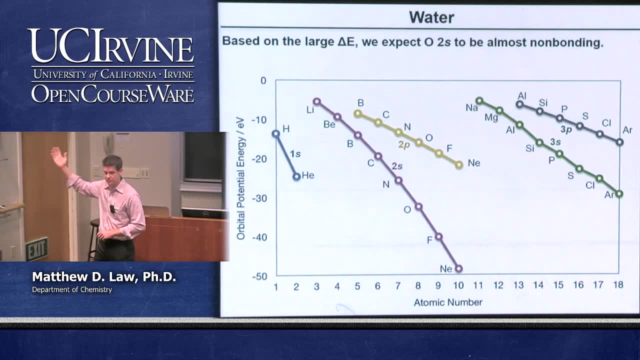 Okay, All right, So we should have some bonding, some non-bonding And some anti-bonding in this particular molecule. We can go back and again remember what the relative energies are. for the atomic orbitals, We need oxygen and hydrogen, which we've already done, of course. 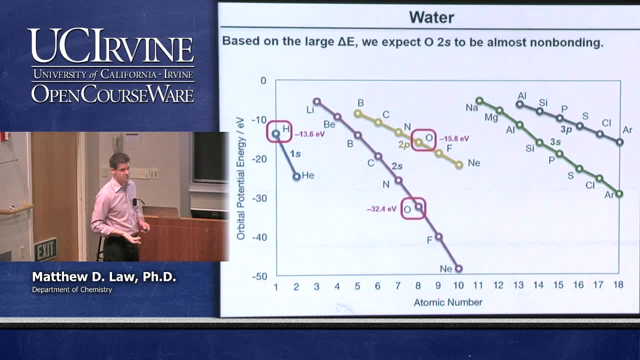 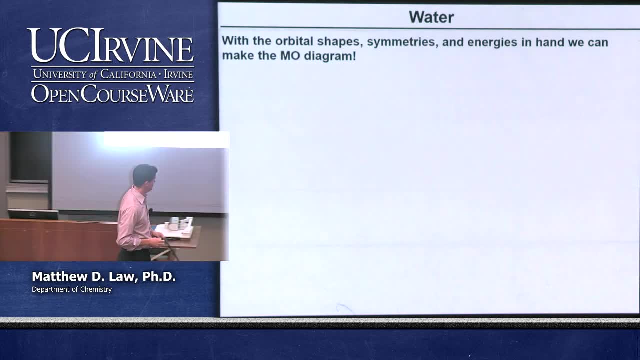 And the thing to remember here is that the oxygen 2s is deep in energy. It's not going to interact substantially with the hydrogens. Okay, So the main interaction is here. All right, So here we go. So let's build the MO diagram. 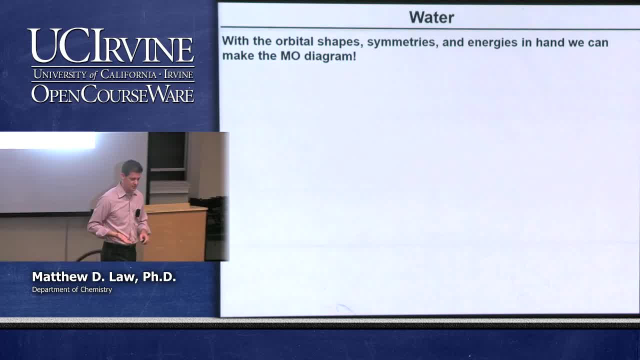 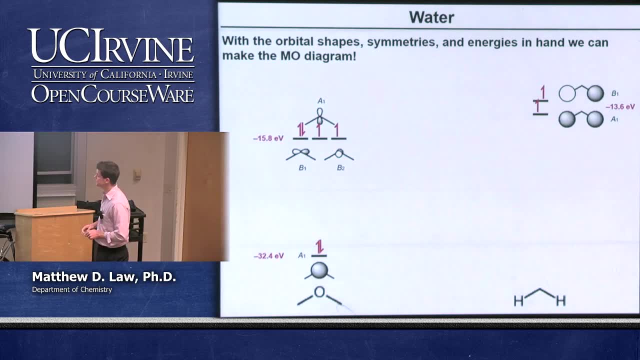 We always put again the center atom on the left, The group orbitals on the right. So here's the center atom. oxygen We can draw it just as the oxygen with, you know, the two bond poles coming out, but not showing the hydrogens here. 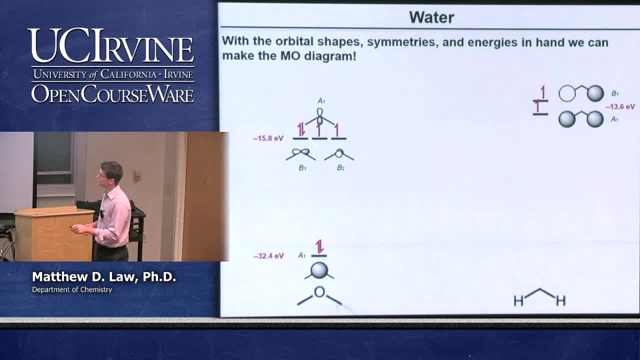 We have the S, which is the A1. And we have the three P orbitals, B1,, B2, and the other A1. And then we have the hydrogens, up here at negative 13.6.. These are identical in energy, to start with, 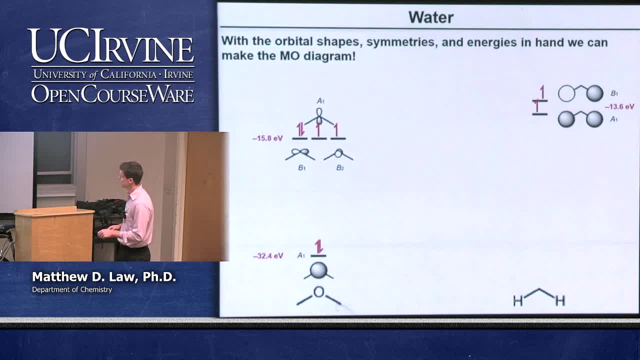 And one is A1.. One is B1. And then we indicate that with the two hydrogens, with nothing at the oxygen position. Now let's build our MO diagram, starting with sigma interactions, All right, And starting at the bottom. What we first expect is basically a nonbonding orbital to come across here, because this guy is so deep in energy compared to the group orbitals. 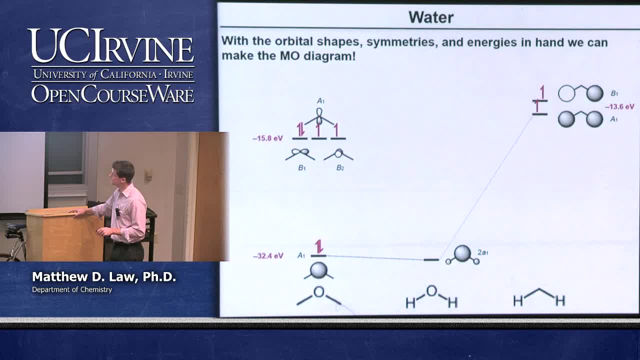 Okay, And so you're going to describe it as mostly on oxygen, with maybe a little bit of tiny character from the hydrogens, And it's all bonding Okay, But it's essentially a nonbonding orbital. So that's one of the A1s. 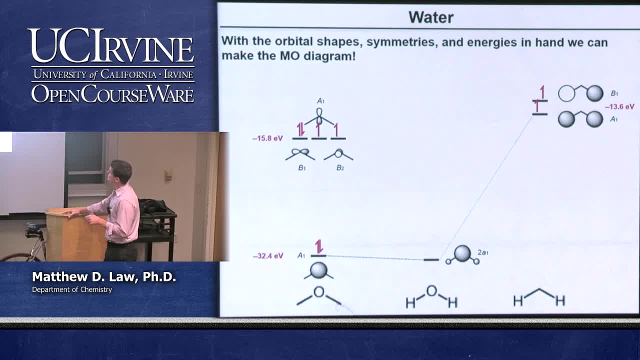 It's just going to come over. The other A1 interaction is between this group orbital and the Pz orbital, And so that's going to give you a substantial interaction, bonding and anti-bonding. And what I've done here is I've just decided to change the shading of the group orbital rather than the center atom orbital. 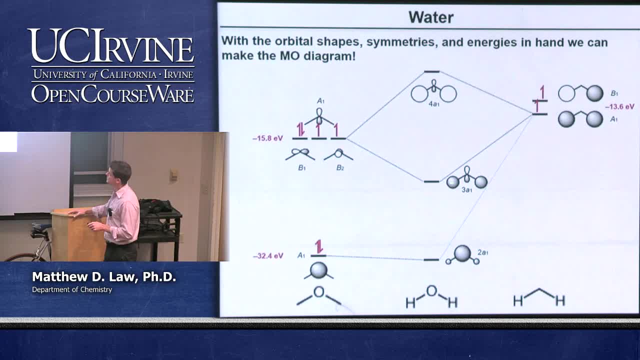 But it's equivalent. You could do either way. All right, This is going to give you Remember. this is pointed in the screen, so it's coming down. So there's a substantial positive interaction here, And then this one has a substantial negative interaction. 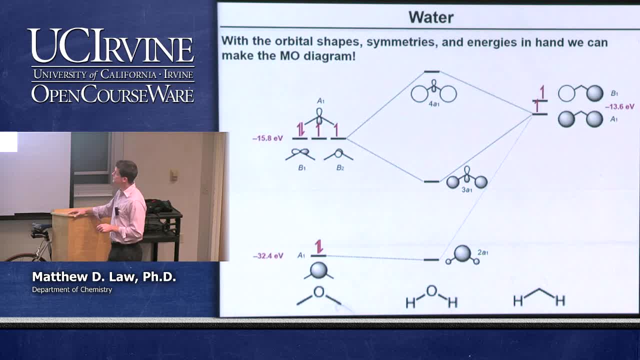 That's why it's an anti-bonding orbital. Okay, These are all A1s, And so we'd label them 2A1,, 3A1, and 4A1.. The 1A1 is with the 1s orbitals. 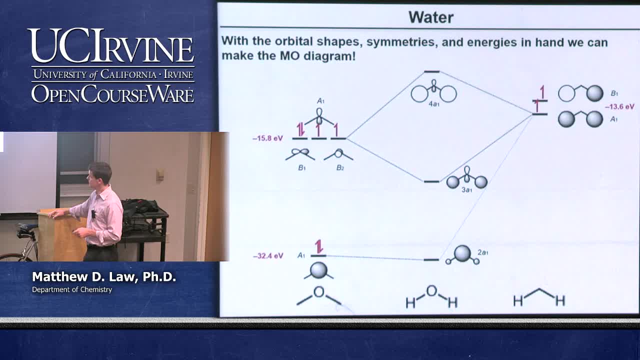 Right, Deeper in energy- Not on this diagram, because we're only looking at valence orbitals. So that takes care of our A1s, Okay, Our three of our six molecular orbitals that we need to build. What about the other interaction? that is actually a real interaction. 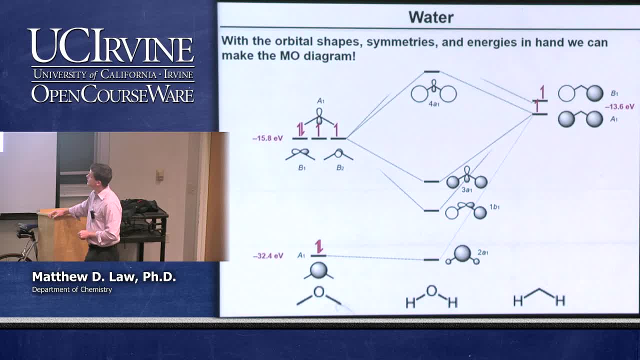 Well, that's the B1. Right, So we have a B1 here and a B1 here, And we draw it in like this. So this B1 is actually going to lead to a fairly substantial sigma interaction, Because The p orbital is pointed toward the 1s orbitals. 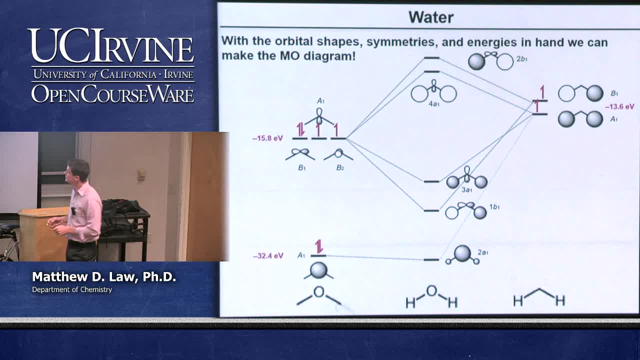 Pretty nicely. It's not perfectly in line, of course, because the molecule is bent, But that's why this interaction is going to be a little bit stronger than this one, And so you're going to have a little bit bigger spread in the bonding and anti-bonding energies. 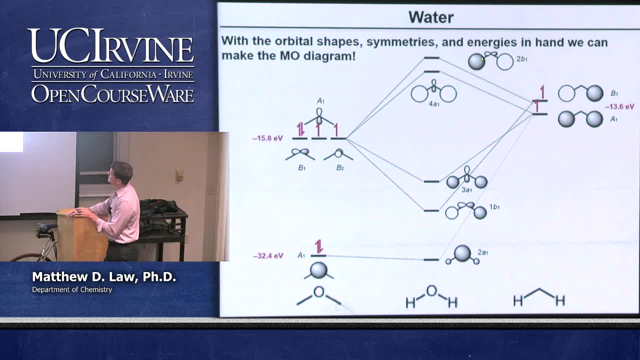 Okay, This is bonding, And then the flip would be anti-bonding. Okay, And again, what we've done is we've flipped the group orbital instead of the center atom orbital, But it's up to you to choose which one you want to do. 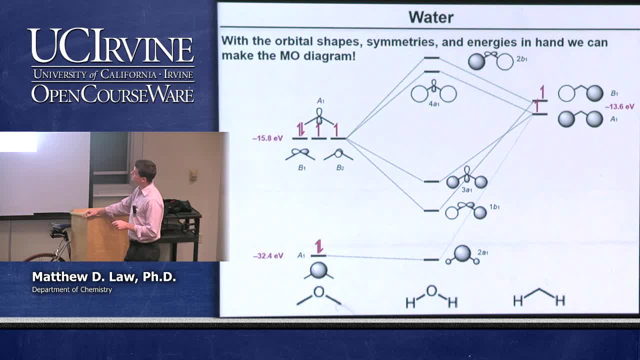 So that gives us two more. So we have only one remaining. Right: We have five molecular orbitals. so far We have only one remaining, That's the B2. Right, The pz orbital, Which has no pair, No partner. 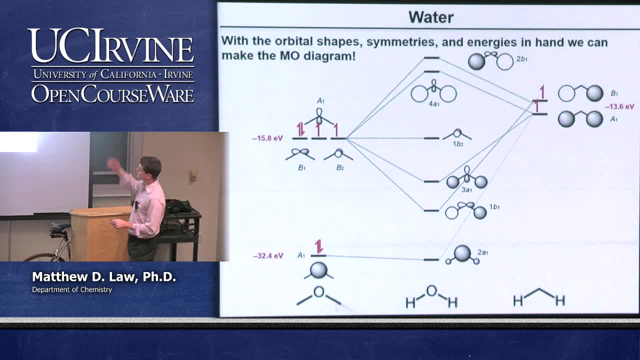 And so it just comes right across, And we label them in numerical sequence according to their irreducible representation. Right, So 1B1.. 2B1.. There's only 1B2 in this MO diagram. Okay, And so that's it. 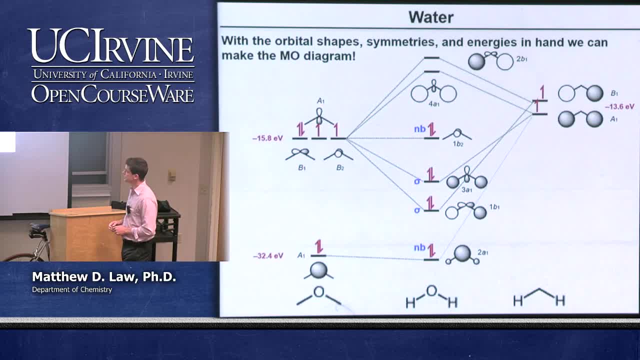 Now we fill it up, Right. So we have eight electrons to deal with with water, Right, And they fill like that. And I've assigned the character of the different orbitals, And so what you see here is that you have two sigma-like bonds. 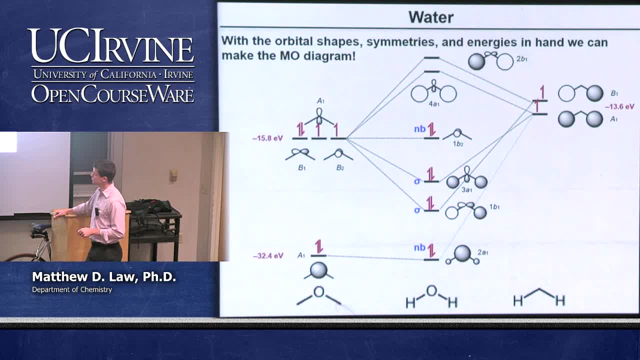 And you have two non-bonding: One that's almost totally non-bonding and one that's rigorously all non-bonding Because it has no symmetry pair, And so this matches quite nicely again with the Lewis dot picture that we would expect. 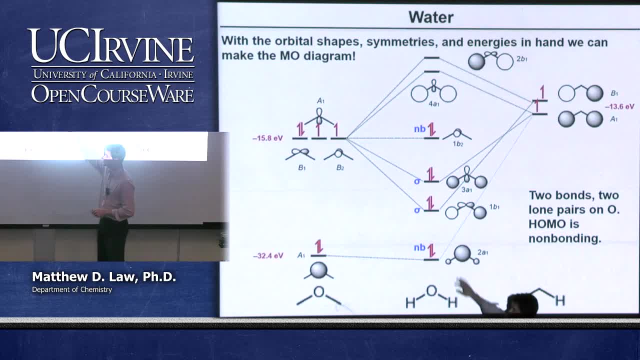 Especially considering that the non-bonding here is primarily on oxygen Right. So that's one lone pair on oxygen, The other lone pair is totally on oxygen. So those are oxygen's two lone pairs, And then we have two sigma bonds. 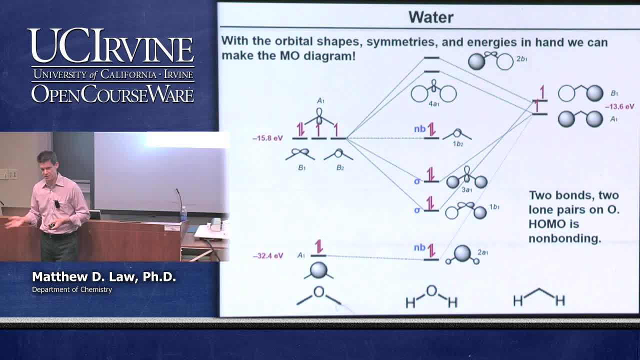 One running to one, hydrogen, you know, in the Lewis dot picture, The other to the other, hydrogen, In the MO picture. again, it's more nuanced than that. Both of the sigma-type orbitals right are interacting- all three atoms at the same time. 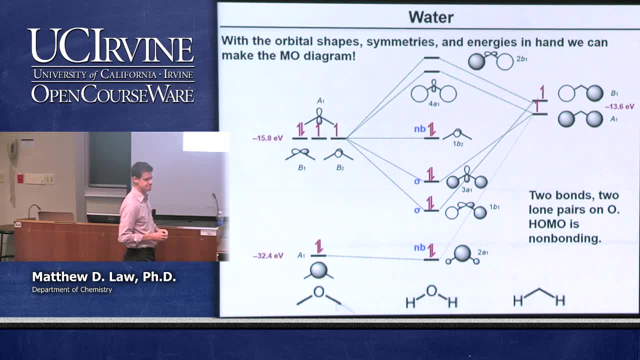 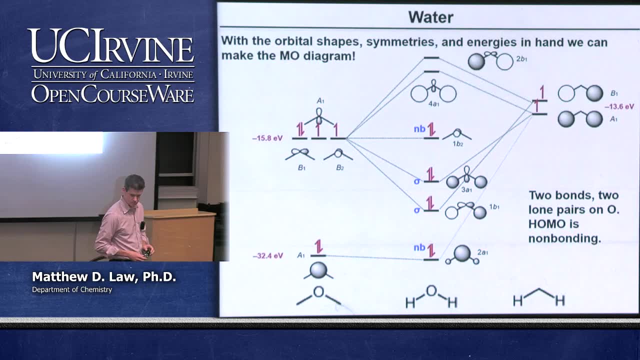 And they have different energies. So again, they're not equivalent. Yeah, So do we consider anything that has a symmetry match, to have even a little bit of bond, A little bit of bonding character, Like the, for instance, the bottom non-bonding orbital? 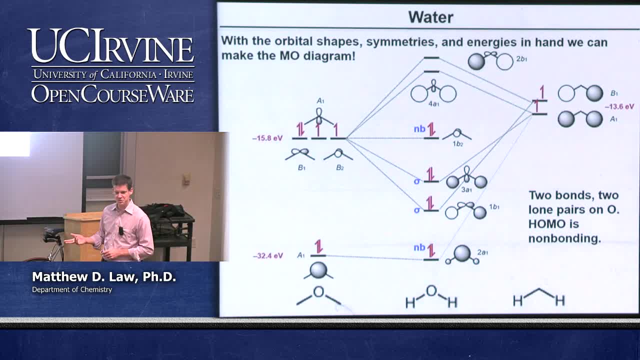 Yep. So this would be, you know, let's say, 95% non-bonding, 5% bonding, So it's almost totally non-bonding, And that's because of the symmetry. No, the symmetry match allows you to actually have the interaction. 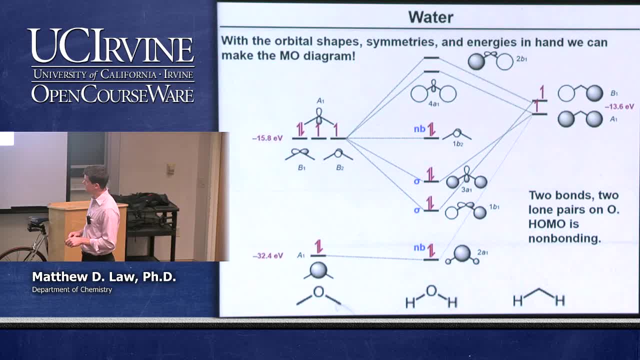 Right. The reason that it's almost totally non-bonding is because this original atomic orbital is so deep compared to this one, So the energy difference is just too large to have a substantial interaction. But you will have, It's not rigorously zero. 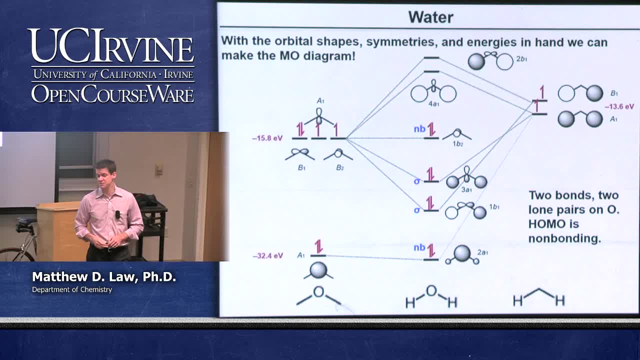 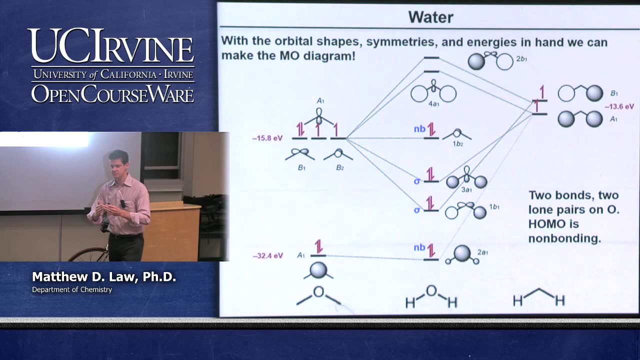 Right. So it's only rigorously zero when symmetry says that there can be no interaction. Other questions about water? So a nice clean MO diagram, Right, Okay, This was our first example of a non-linear molecule. We again had two group orbitals that we needed to worry about. 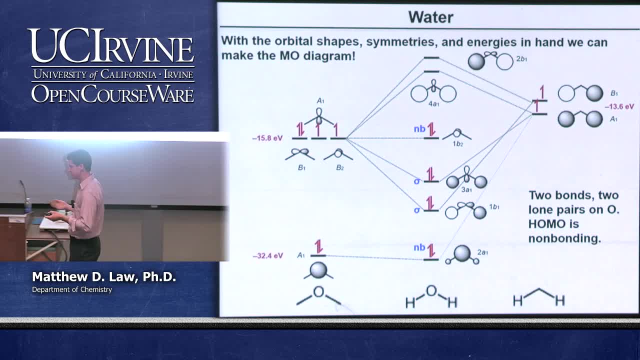 We just had two 1s's in this case, So again we could do it sort of fairly easily. We could build up what the group orbitals must look like Just by taking their sum and their difference. But this is not always possible when we start talking about molecules that have more than two atoms in the group orbitals. 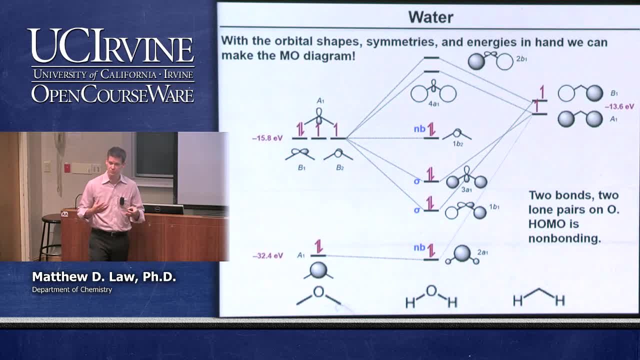 It becomes non-trivial to figure out how to build the atomic orbitals into the molecular orbital, And we're going to see this in the example that's next. BF3 is what we're going to look at next. Okay, So we're actually about a lecture behind schedule. 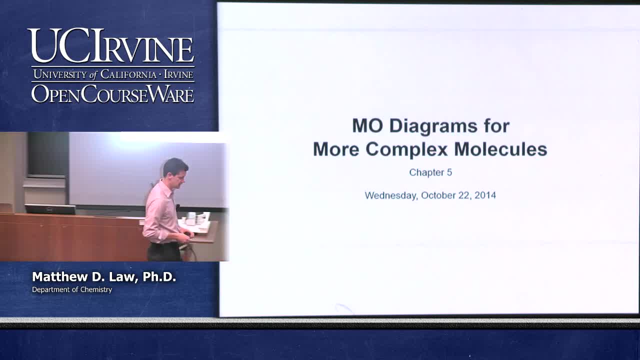 Which is fine. It just means that we're going a little bit more slowly. This is, in part, because there are lots of good questions that are being asked, So I totally encourage that. So please continue to ask questions. Slower is probably better with this material. 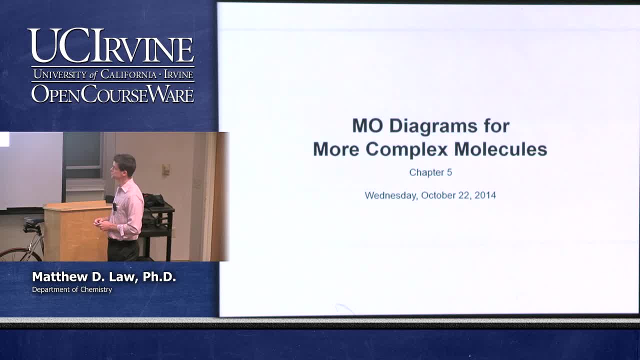 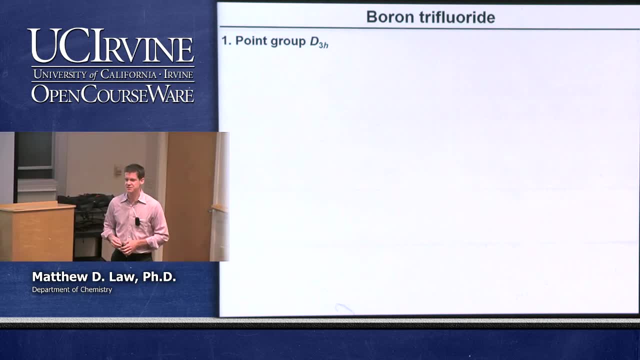 Okay, So this should have been Wednesday's lecture, But we'll do most of this lecture today. Okay So boron trifluoride. Why is this a good example? It's because it's a nice planar molecule with more than two outer atoms. 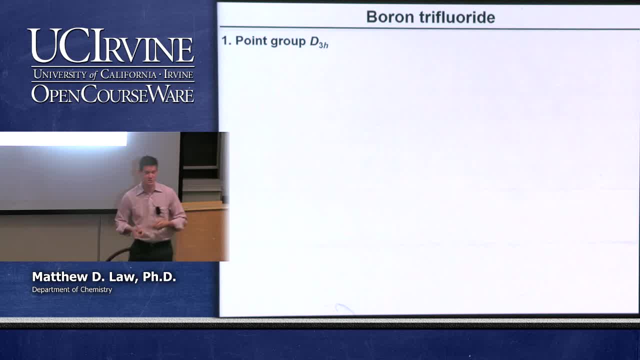 So we have three outer atoms now, And this introduces a new concept that we need to understand in order to build molecular orbitals from these more complex molecules. The procedure is essentially the same. What we're going to do is introduce a new idea on how to actually build the molecular orbital wave function. 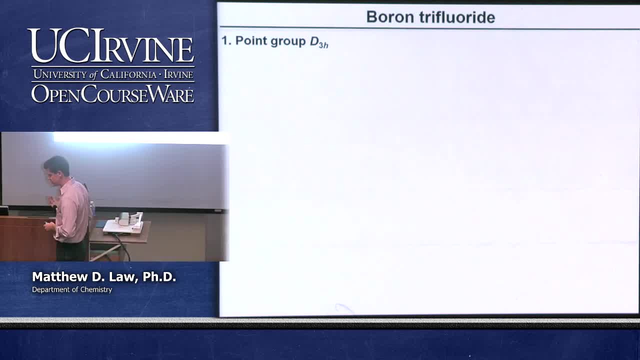 Essentially the shading diagram. Okay When the time comes, But up until that point our procedure is exactly the same. We select what the point group is for the molecule. In this case, boron trifluoride is a planar molecule. 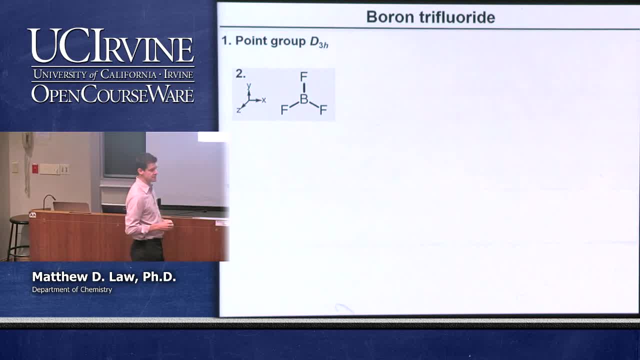 So it's D3H. It looks like that. Right, We assign its Cartesian axes, And remember that the convention that we're going to use is we're going to use the z-axis along the main rotational axis, And then the y-axis of all the outer atoms are going to point toward the central atom, if there is one. 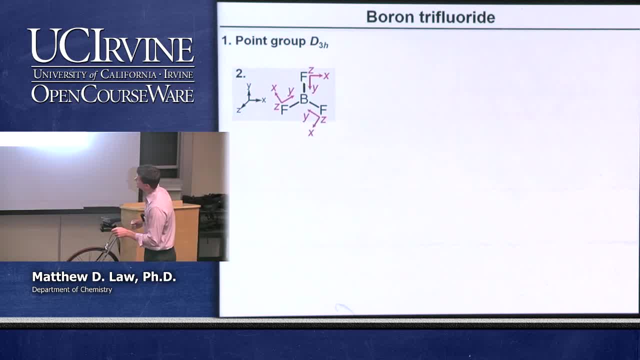 Okay, So we assign different Cartesian coordinate systems for each of the outer atoms, Each of the fluorines in this case. The y-axis are always pointed toward the center atom. The z-axis are coming out at you, So that gives us our geometrical problem. 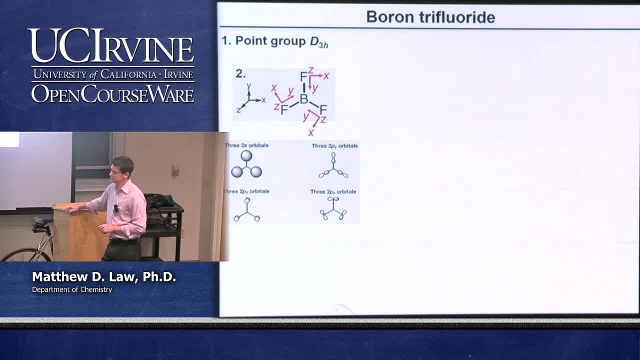 And then, of course, the nice thing about fluorine, or maybe the complication with fluorine, is that you don't have just 1s orbitals anymore you need to worry about, But you have s and p orbitals. So this example here has s and p from the three outer atoms and s and p from the center atom. 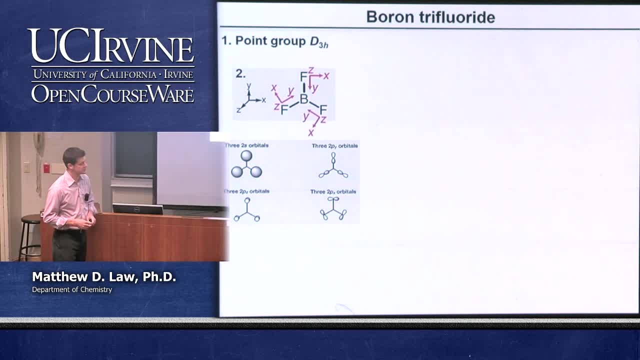 So it's a little bit more complicated than, for example, if you used ammonia. Right, If we just did ammonia, we'd only have to worry about 1s outer atom orbitals. But we've got s, We've got the three p's. 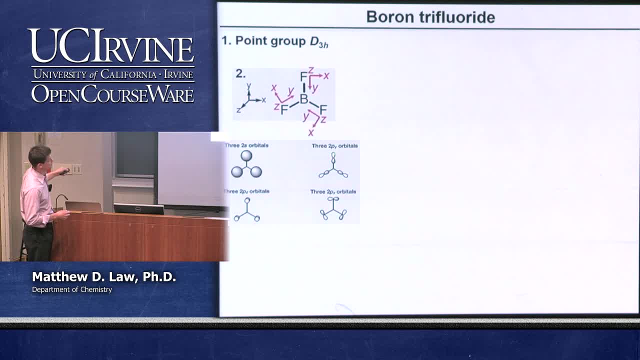 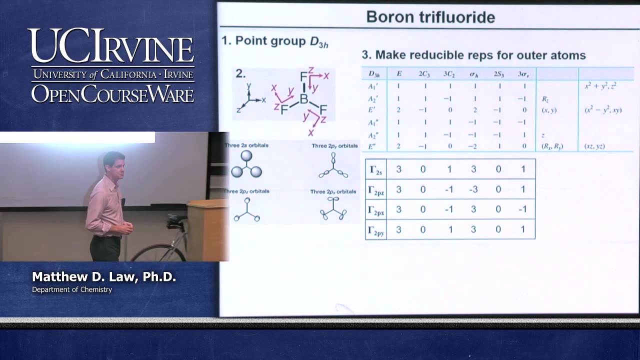 And with these Cartesian coordinates, this is how the three p's would be drawn: Py's all point toward Pz's coming out at you, Px's orthogonal to the other two directions. Okay, So that's how they would look, And what we want to do is select the reducible representation for each separate kind of atomic orbital. 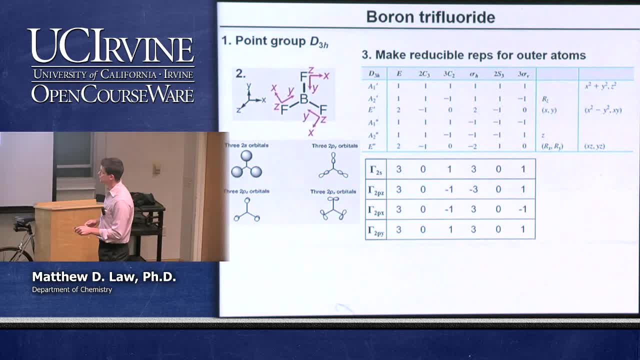 S, Px, Py and Pz, And so we can build our reducible representations for each one of these. You can convince yourself, for example, that for the two s's, if you just stare at this Right Under E, it's a character of 3.. 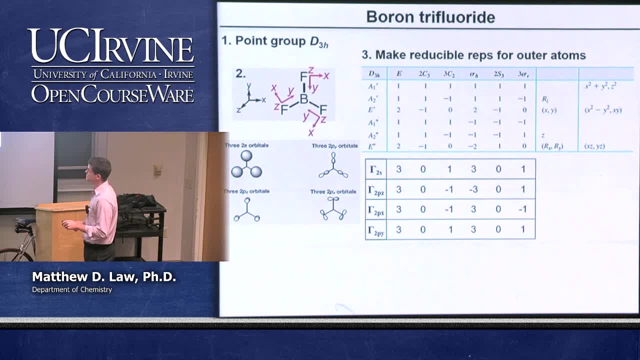 Under a C3, all of them move, And so it's a character of 0. A C2 axis. there are three of those. One passes that way, One passes that way, One passes that way. Upon 180 degree rotation, two of the orbitals move. 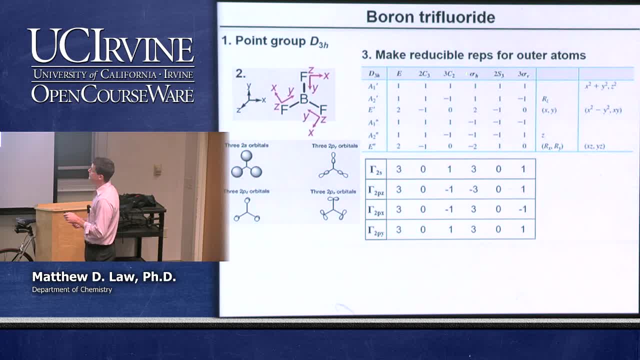 One does not, And so that gives you a character of 1. The horizontal mirror plane. nothing moves. Character of 3. And S3, all of them move, And a vertical mirror plane passes again through, always one of the outer atoms. 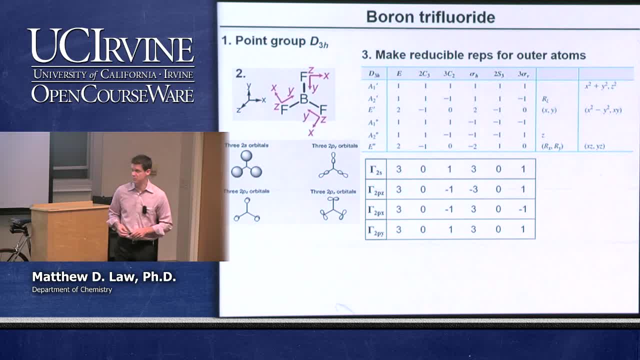 And so one of them doesn't change and the other two flip. Okay, And so that's how we build the reducible representation for the two s's, And you can do the same thing for the other three. So we build the reducibles. 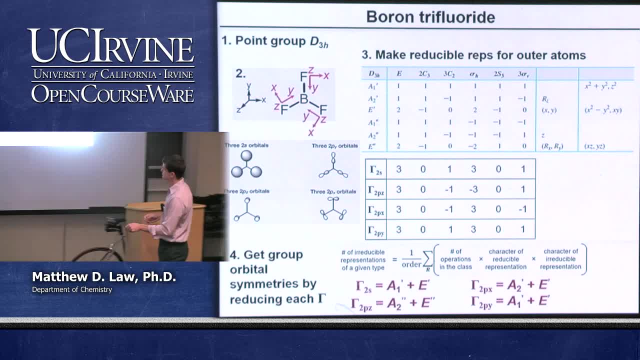 We reduce them, And when we reduce them, we get these results here. Okay, You know a six by six character table now, So you would, in principle, have to go through all six and assign how many of those are in each of these reducible representations. 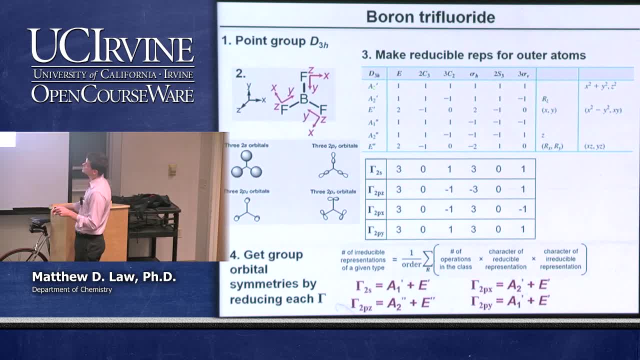 And it turns out that the two s has an A1 prime. You can see we've got an A1 prime kind of label here. There's an E prime because there's two different kinds of Es: E prime and E double prime and so forth. 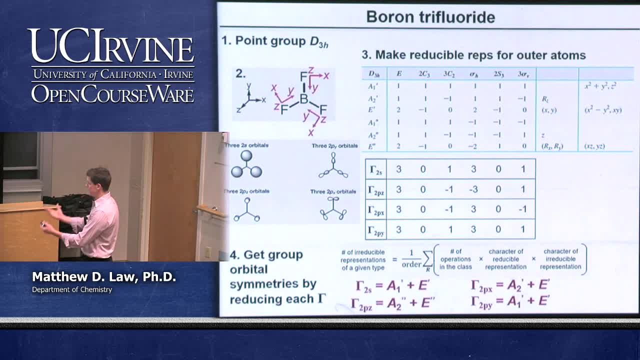 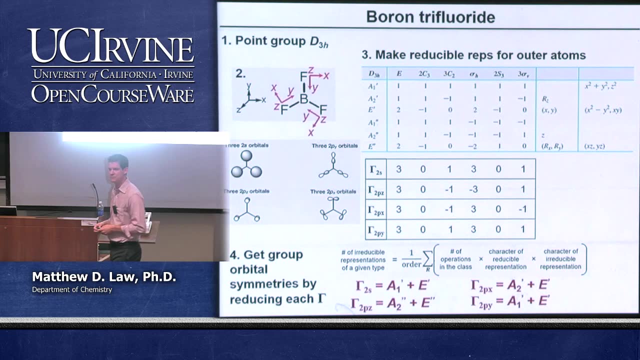 Okay, So we have now assigned the symmetry of the individual groups, The individual group orbitals. Okay, From all of the s and the p's from the outer atoms. What we want to know next is how do we actually build them in our shading diagram kind of scheme? 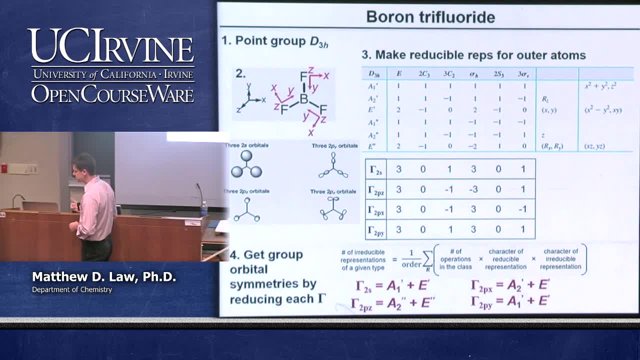 What do they actually look like? Okay, One thing to keep in mind here- and this is also the first example of this phenomenon- is that we have now E right Irreducible representations. Remember when you see E. this is a two by two matrix. 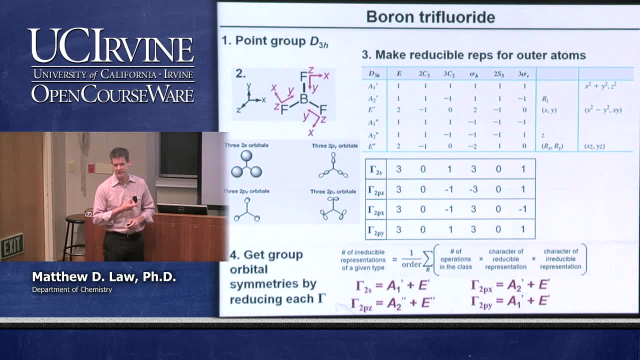 And so this means that there are two orbitals That are in that E, That have the E prime symmetry. Okay, And if we look at what E prime symmetry says here, E prime symmetry says that we go as the x and the y coordinates. 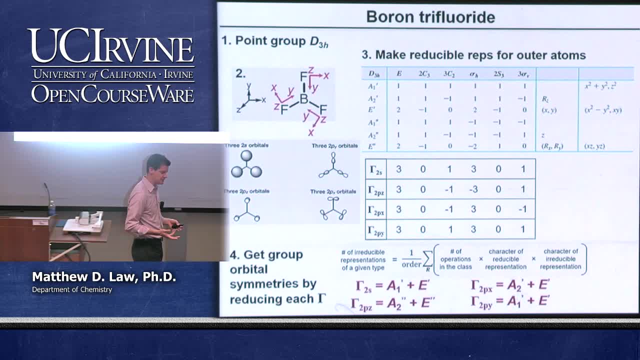 And so we expect one of the orbitals in the E prime set to be x like, And one of the orbitals in the E prime set, the other one to be y like. Okay, Y like symmetry, And we'll see how this plays out. 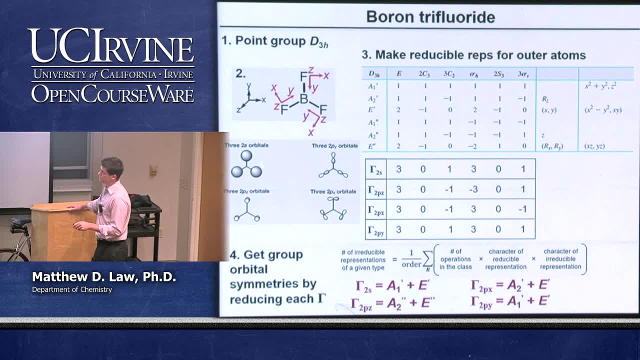 But just keep in mind, as it must be true, Right, We have three outer atom 2s orbitals, So there must be three irreducible representations Or three orbitals in the irreducible representations. One here and two here gives us three. 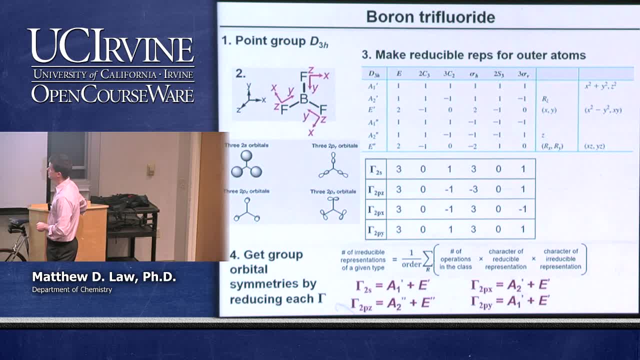 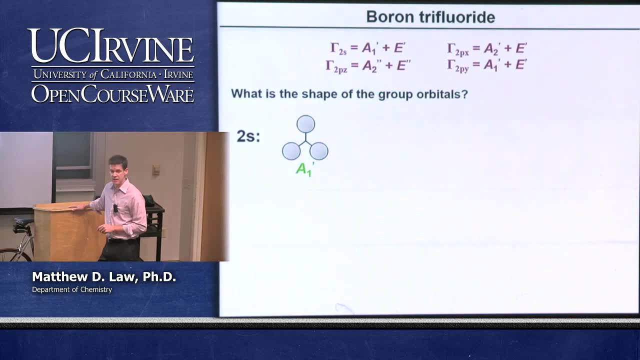 And that's the same for all the other orbitals as well. So let's look at the 2s's And try to understand how we can construct what the shading diagram should look like for the wave function For the 2s's. we have these two. 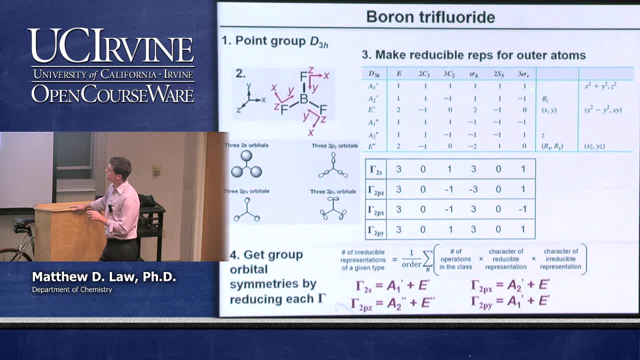 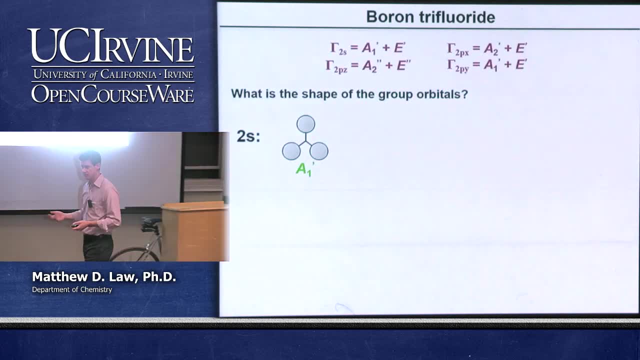 Okay, The 1 prime, if we look at it, is the totally symmetric representation, And so we know right away how to make that one out of s orbitals. It's just taking the three s orbitals, all of the same sign. 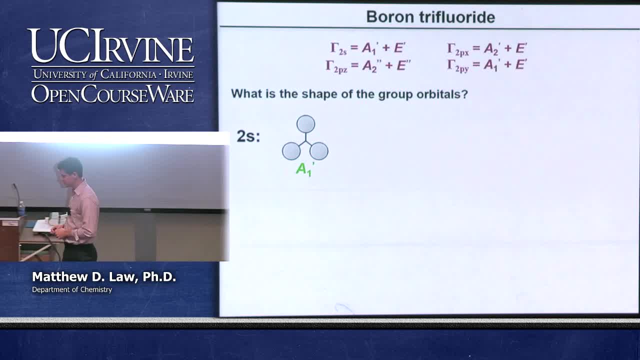 Okay, That's the totally symmetric representation, So we can just immediately guess what that one's got to be. So it's got to look like that. The question is for the other two that are buried in the E prime: what do they look like? 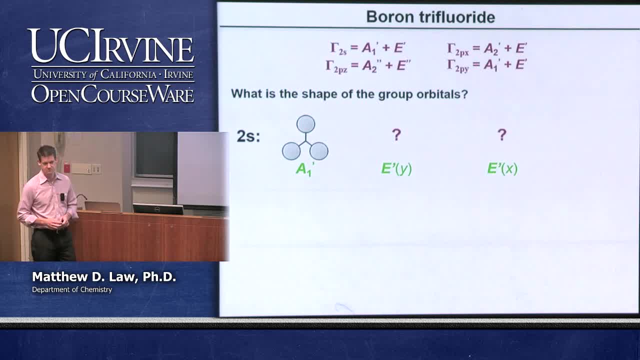 And you can see the problem. We can't just take the difference, Because you're taking the difference of what You have- three things now that go into a linear combination. So we need a procedure that allows us to properly select the right linear combination to give us the correct symmetry. 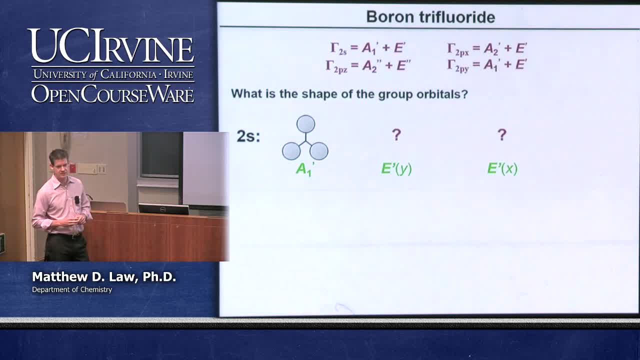 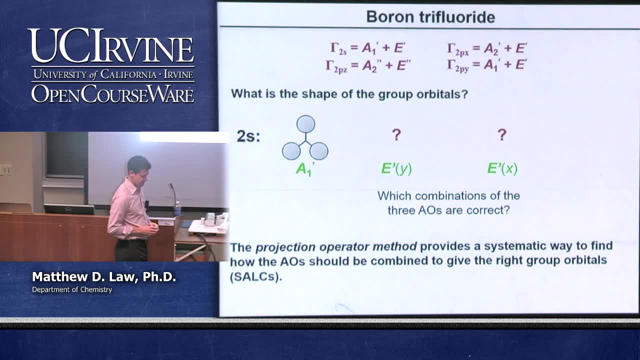 Symmetry that matches the E prime for the Y and the E prime for the X, And the way that we do this- this is described in your book, of course- is the so-called projection operator method, And this is the last big concept in chapter 5. essentially, 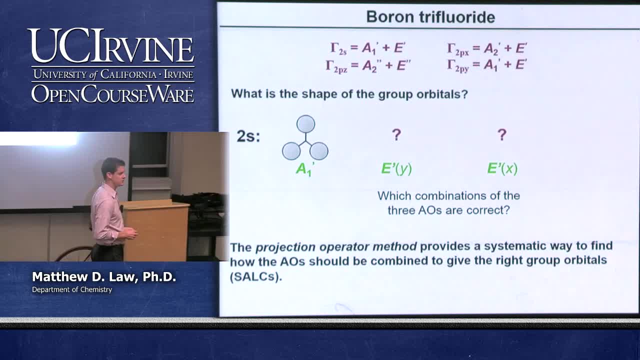 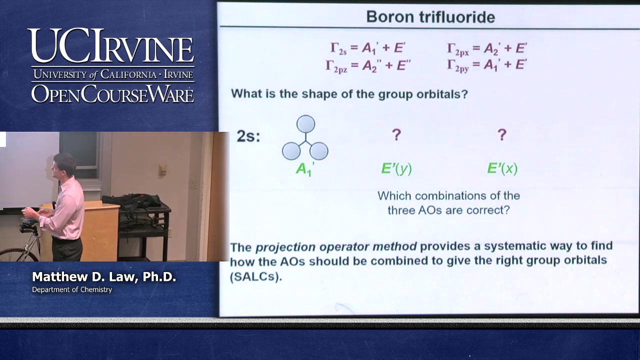 This is the mechanism that we can use, the machinery that we can use to construct the molecular orbital wave functions. When we have some sort of ambiguous situation like this, We don't really know how to do it, just by looking at it. So the projection operator method gives us a systematic way to find out how the atomic orbitals should be combined to give us molecular orbitals that have these symmetries. 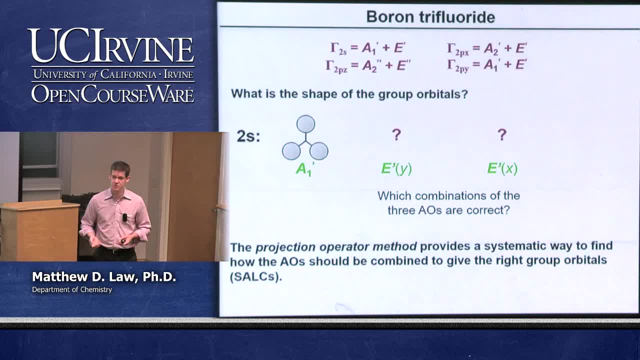 So it's a technique that comes out of group theory. We're, again, not going to derive it, We're going to use it. We're going to just use the machinery. So let's look, We're going to start at trying to understand how we can build the E prime with Y like symmetry. 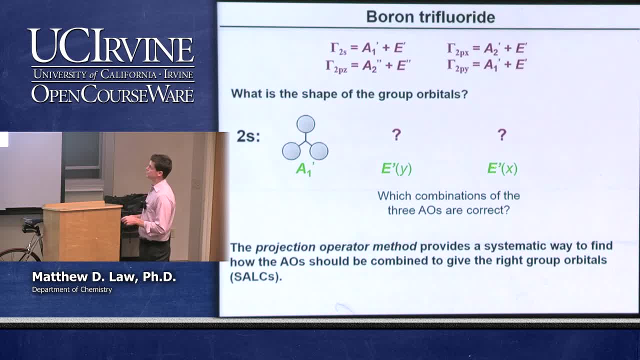 And it turns out that the projection operator method is not going to be able to give us both of these. It's only going to be able to give us one, And so we're going to get this one from the projection operator method And we're going to get the other one from normalization and orthogonality. 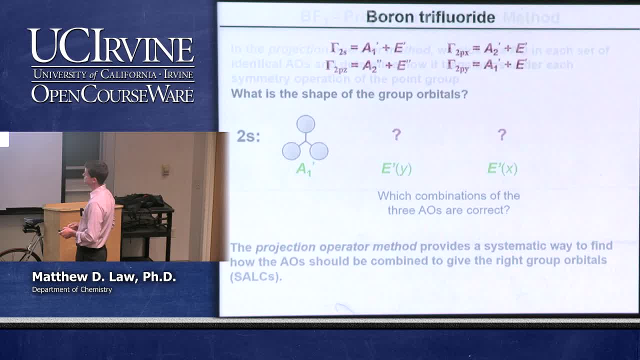 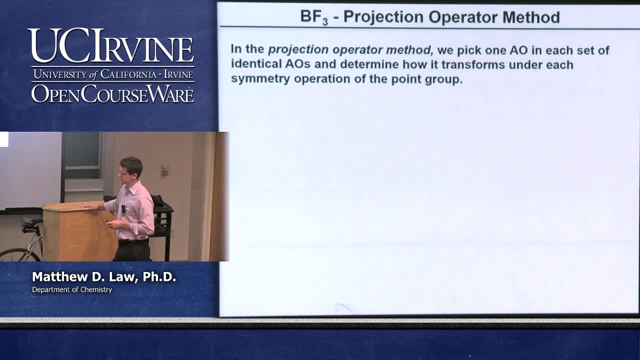 Like we've discussed in the character tables before. Okay, So what do we do in the projection operator method, The basic procedure? Again, it all boils down to procedure, because we're not deriving the method itself. We pick one atomic orbital in each set of the identical atomic orbitals. 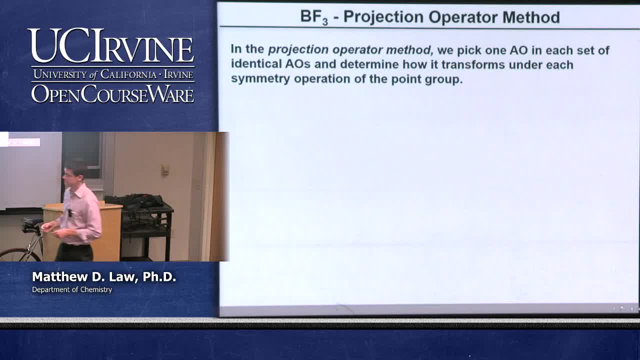 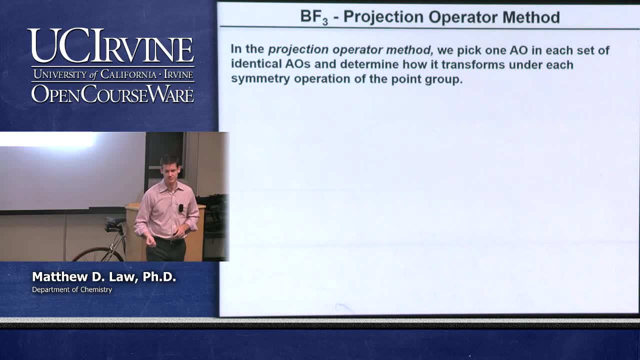 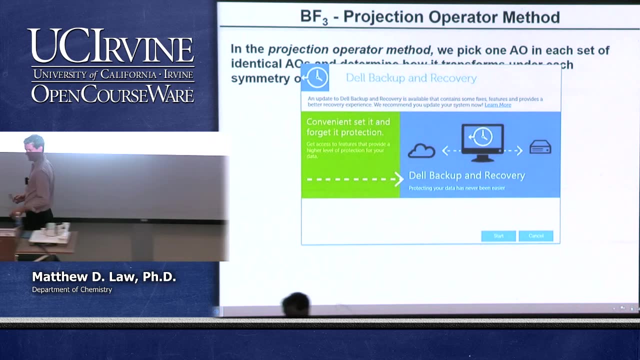 So, for example, we pick one of the 2s orbitals- is what we're going to do- And we determine how that orbital transforms under each of the symmetry operations, Every single symmetry operation in the point group. Somebody pressed their button on the remote. 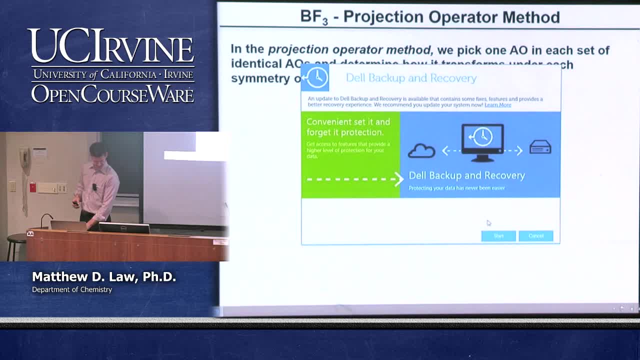 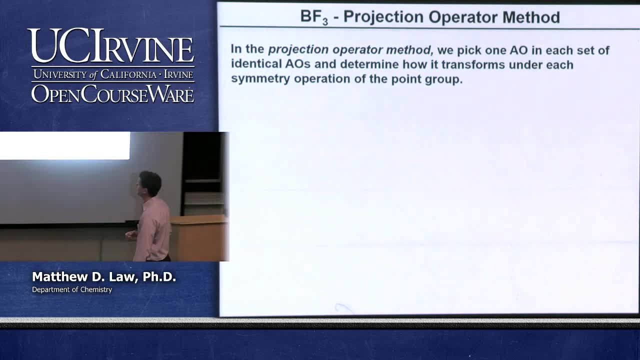 Let's see here. There's demons in the computer this morning. Alright, Okay, So how does this work? What we do is we're going to look at the 2s's right, Because that's what we're interested in right now. 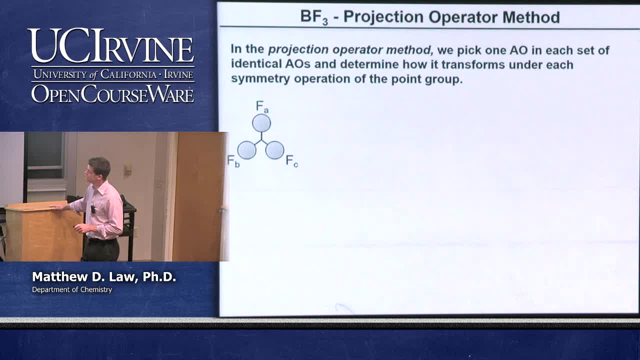 We assign labels to each of the fluorines A, B and C. Okay, And we're going to look at fluorine A here, We're going to do the symmetry operation And we're going to figure out what fluorine A turns into. 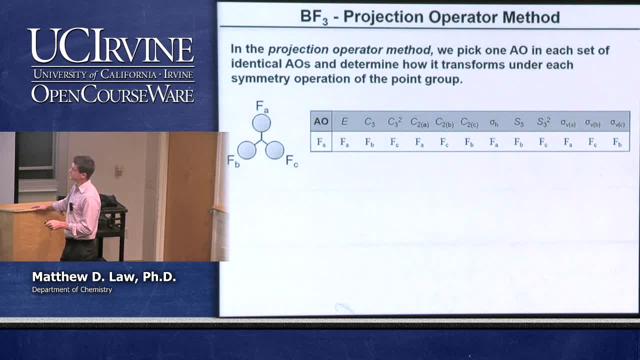 So here's how we do it. The atomic orbital that we're considering is fluorine A, And these are all of the symmetry operations spelled out from the character table, The D3H character table. So if we do nothing, F A remains F A. 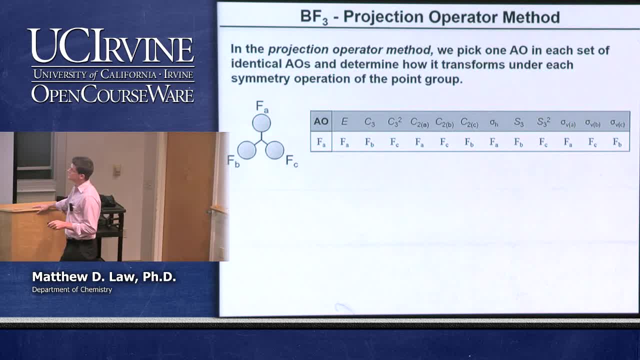 If we do a C3, remember we're doing counterclockwise rotation, So F A becomes F B. That's what we're saying there. If we do that twice, F A becomes F C. Goes to the F C position. 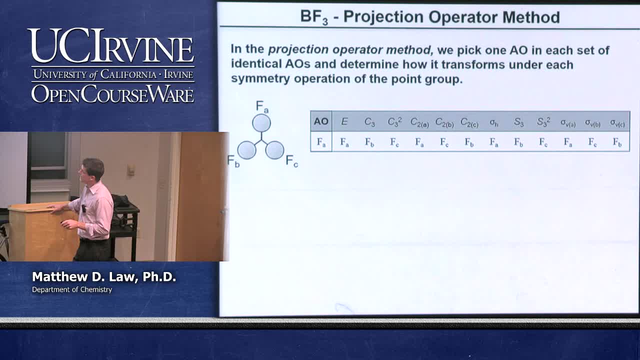 If we do a C2 along the A axis, That's the axis that passes through atom A here, Then F? A remains F A. If we do it along B, then F? A becomes F C, And et cetera, et cetera. 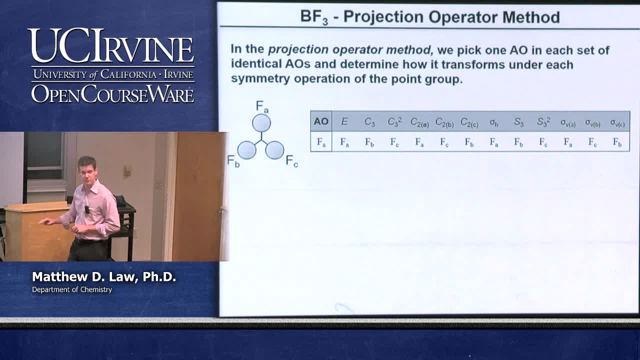 We do a horizontal mirror plane reflection, F A stays put And we just run through all of the different symmetry operations And find out what F A becomes Okay. And we build up this long list here Because we have quite a few symmetry operations to do. 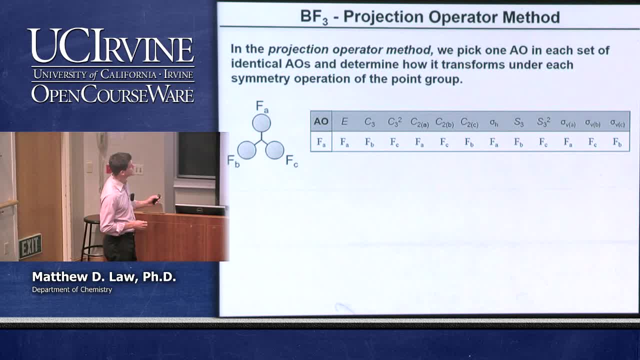 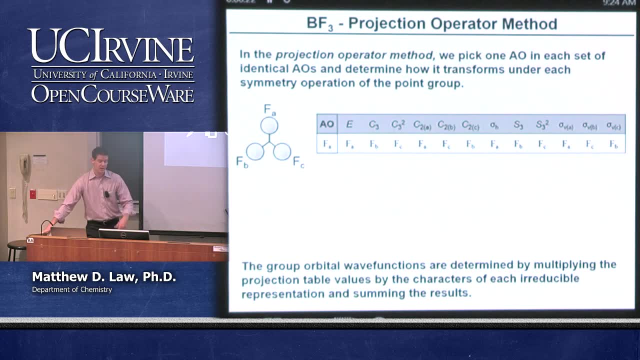 Symmetry operations to deal with in this particular point group. Okay, Let's hope that this continues to work. Okay, So how do we actually take this information and make use of it? Okay, So what we've done is we've looked at an atomic orbital and we've seen how it transforms under every symmetry operation in the point group. 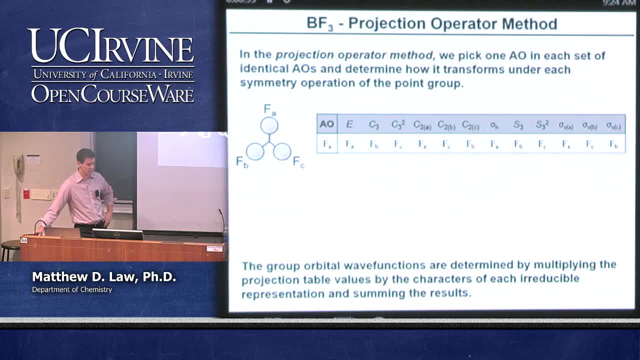 What we want to do in order to describe what the group orbital wave function is going to look like. We multiply these different Results here By the characters in the irreducible representations, Going down from the first one, the A1 prime, through all of the others in the point group. in principle, 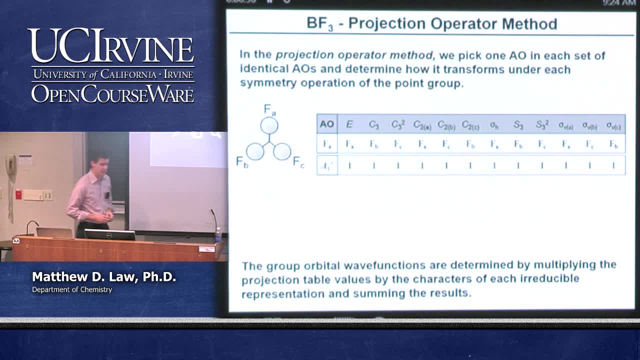 And so what do we do? For example, A1 prime has these characters If we just pull it out of the character table. this is what A1 prime is: Fully symmetric representation. Okay, And we have an A1 prime that we care about, because the 2S is reduced to an A1 prime and an E prime. 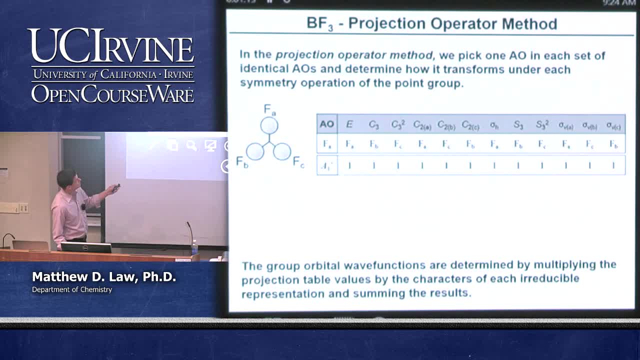 Okay, We multiply the characters. Multiply each of the characters here in each column by the functional form here of the result from our atomic orbital manipulation. So we have 1 times FA plus 1 times FB, plus 1 times FC, etc. etc. 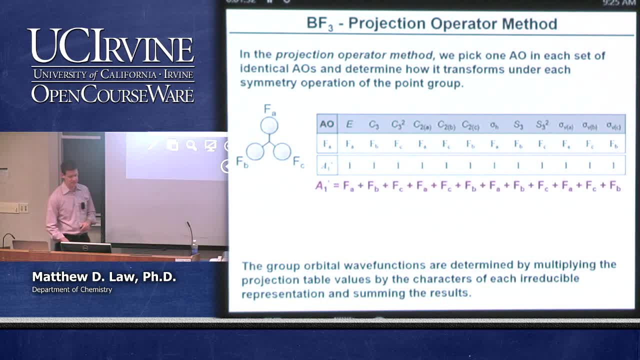 All the way across, And what that gives us in the end is the A1 prime. This is a way to represent the functional form of the molecular orbital wave. function Is going to be equal to FA plus FB plus FC, etc. etc. 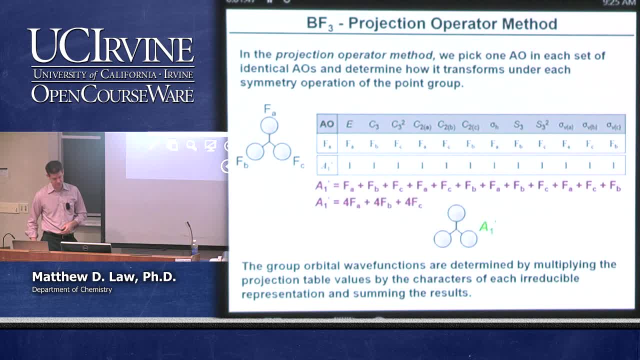 All the way across, Simplify, Right, Collect terms And what we find is that there's 4 FAs, there's 4 FBs and there's 4 FCs. And so we're saying now that the molecular orbital wave function of A1 prime has equal contributions of FA, FB and FC with the same sign. 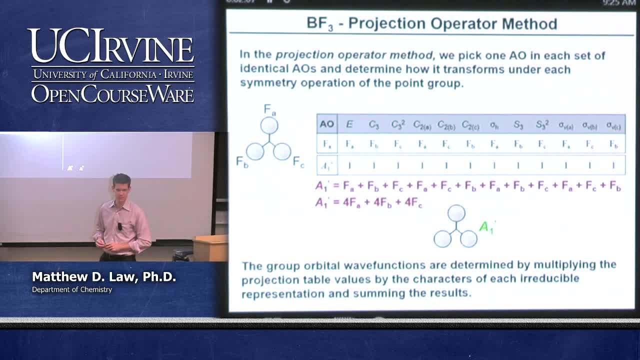 And that's exactly what we just, you know, spit out just by looking at the problem, without considering any of the math. And so the A1 prime has this kind of function to it. That's what the molecular orbital wave function must look like. 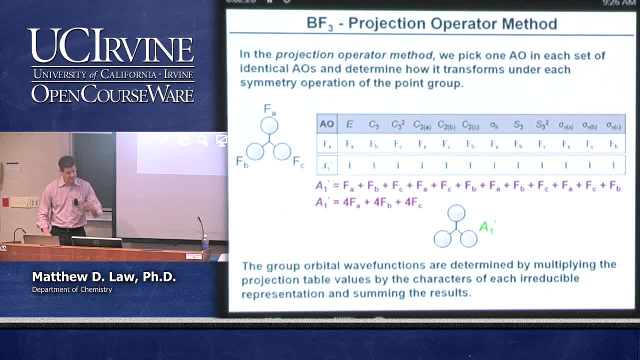 We can then go down the list of different irreducible representations if we want to, in the character table. For example, let's consider A2, prime Of which there is none. There's no A2 present in the 2s orbitals. 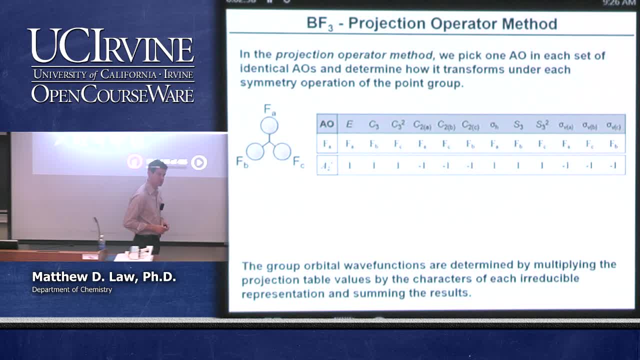 Right, We said that the 2s orbital irreducible representations are A1. And E prime. So if we look at A2 prime, it has these characters. We just pull those out of the character table, We multiply this by that, this by that, this by that and sum up the products. 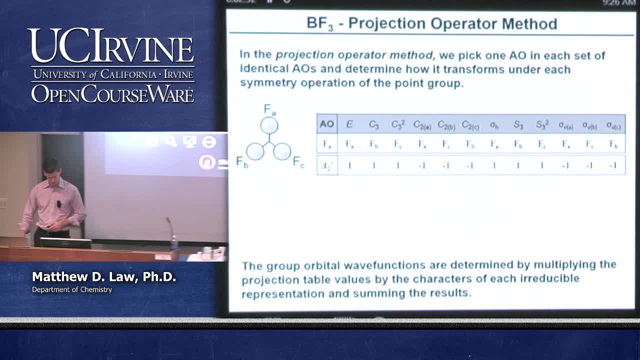 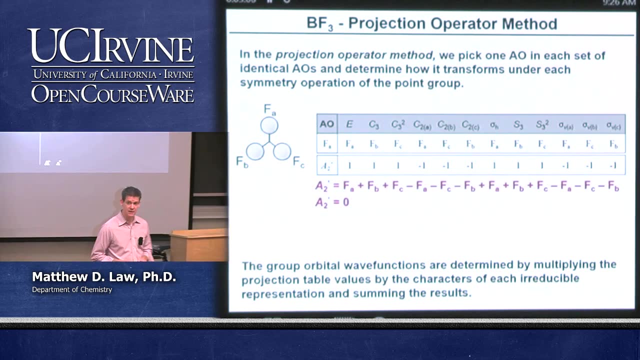 And what we find is that we have a function, that when the terms are collected, we have everything canceling out Right. So all of the positives and the negatives cancel out And we get A2. prime is equal to 0. And what that means is that there is a function. 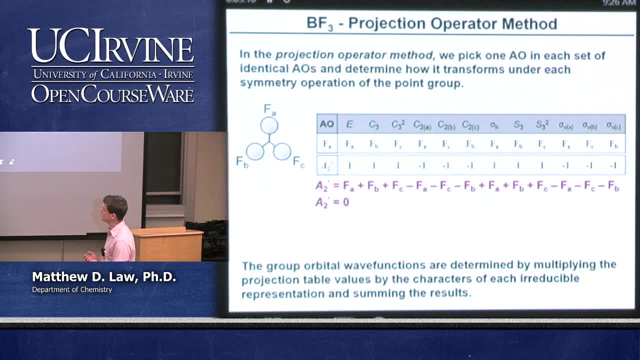 What that means is that there is no function that you can use with these 3 orbitals to build an A2 prime- irreducible representation. In other words, these 3 atomic orbitals don't make an A2 prime, And we already knew that, because when we reduced our reducible representation, we found no A2 prime present. 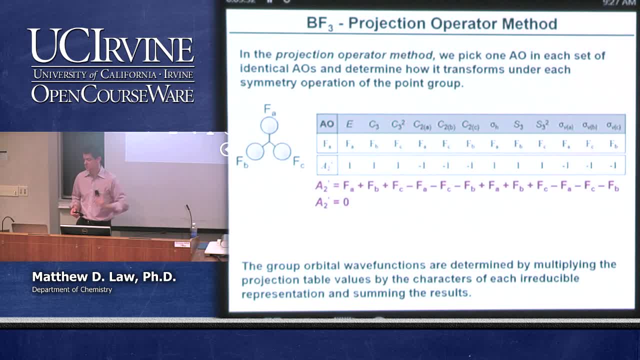 So the projection operator method confirms this result. There is no function that is A2 prime, like from these orbitals. The next one down in the character table is E prime, Which we know from our reducing that it should exist. There should be an E prime. 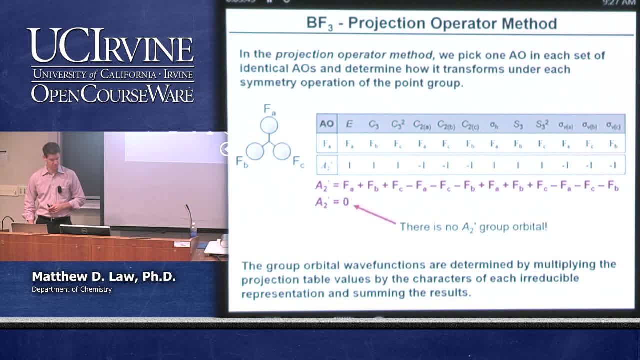 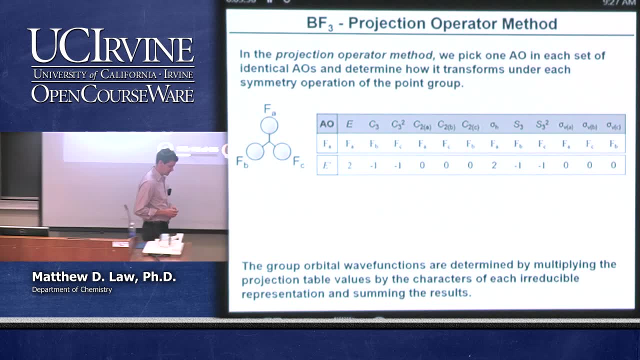 So this tells us, when you have a result of 0, there is no function present with that kind of symmetry. The third and final one that we need to worry about- because we're just kind of marching down the table here, And this is the last one that's actually present in the reducible representation- is the E prime. 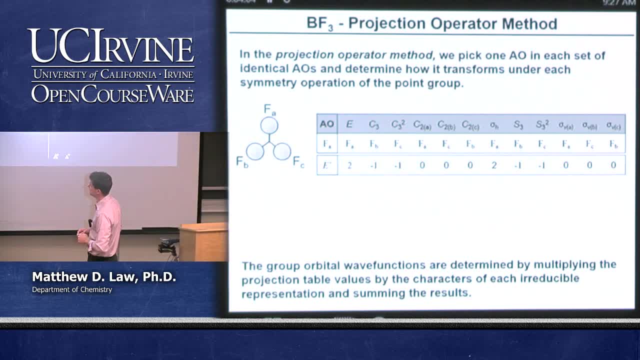 These are the characters for the E prime, just pulled right out of the table, And so we can see that. And so we can see that there's something new here, Because we have the character 2 for E and we have another character of 2.. 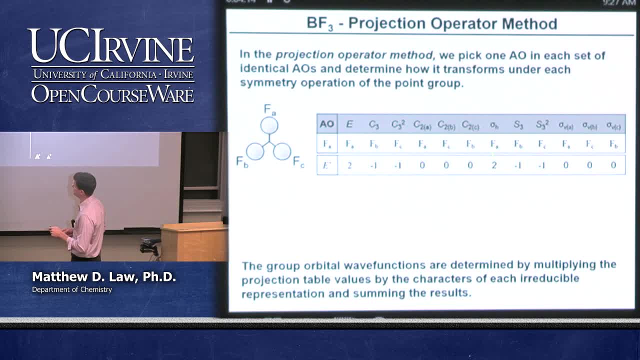 So the FAs are both multiplied by 2. So there's going to be 4 FAs in this particular function. Let's see what the rest looks like. You just multiply and add up the products And what you're going to get is this: 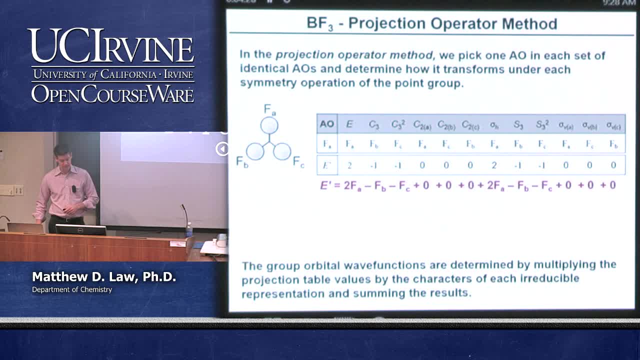 There's lots of 0s in there, so it simplifies pretty easily And if we collect terms, you find that the E prime is equal to 4 FAs minus 2 FAs, Minus 2 FBs, minus 2 FCs. 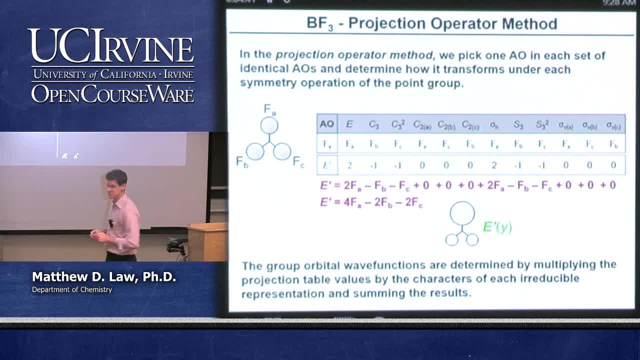 In other words, the contribution from FA is twice that of FB and FC And the polarity of FB and FC- the sign is negative compared to the sign of FA, And so the simple global picture or the shading diagram that we would draw would have FA. 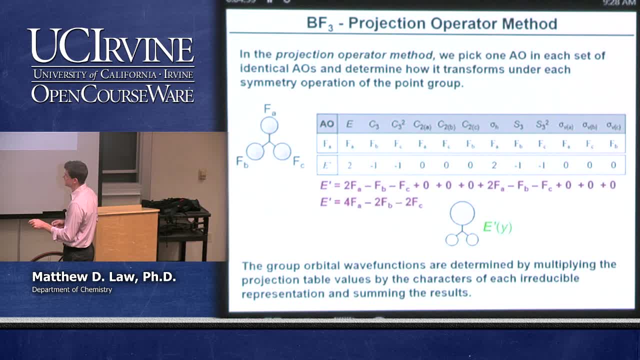 Remember: this is FA, this is FB, this is FC. FA twice that of the size of that of FB and FC And FB and FC having a negative sign, Having the opposite sign of the atomic orbital wave functions. And this just one second. 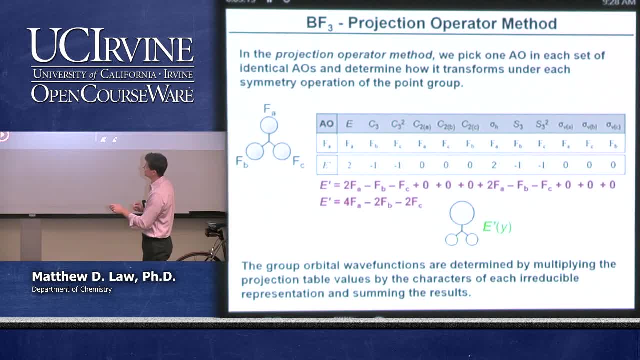 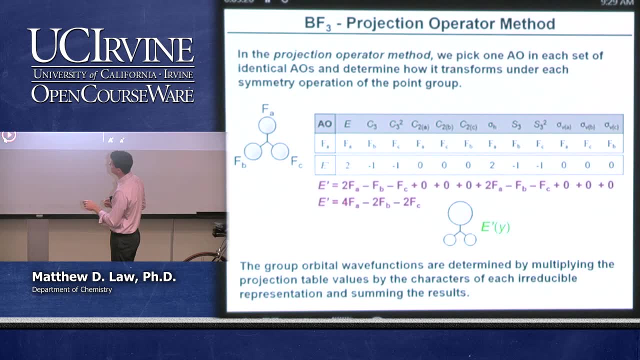 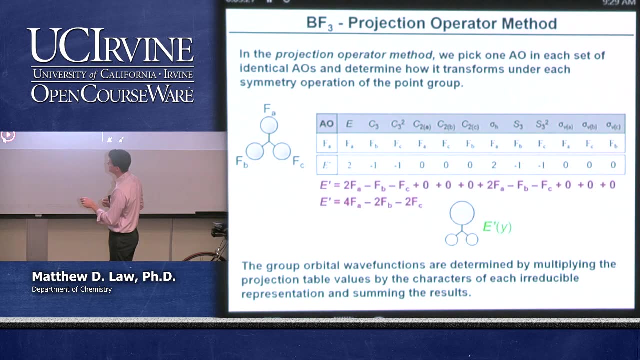 This, then, would give you an orbital that corresponds to the E prime set with Y like symmetry, And what I mean by Y like symmetry is that there is a node that passes right through here, And this is the Y axis, remember. So on one side of that node, the orbital is positive. 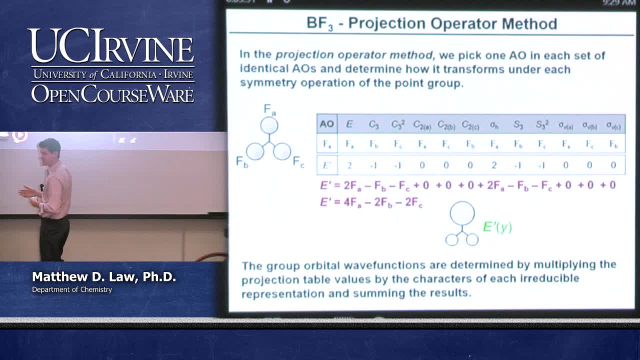 On the other side it's negative, And that's similar to the Y axis. It's positive on one side of zero. It's negative on the other side of zero. Question. I just wanted to double check. You said that the 2S orbital irreducible representations are A1, E and E prime. 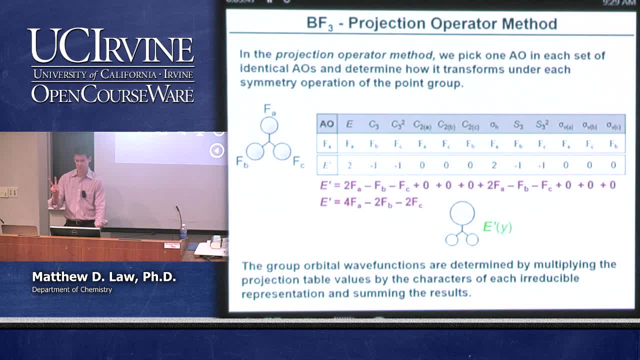 It's A1 prime and E prime, So there's just two irreducibles. One has two wave functions and the other has one. Okay, And so the projection operator method allows us to determine what the functional form is of this particular molecular orbital. 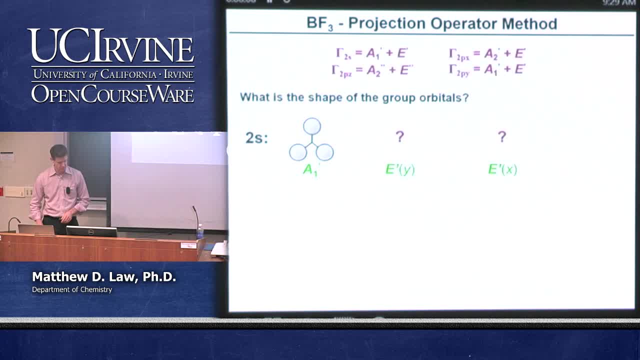 And so we go back to our list, hopefully Okay. And so we were wondering what this one is. We used the projection operator method to tell us that this one looks like that. An important consideration right now we can look at very quickly is that this molecular wave function here must be orthogonal to that one. 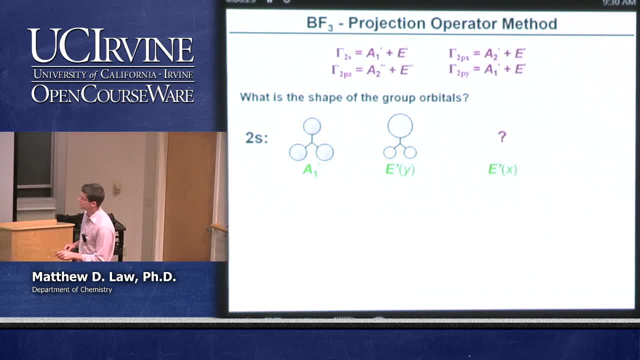 If you multiply the two together, they must equal zero, And you can see that that's going to be true. We're going to have a substantial positive and then an equal and opposite negative, And then when you multiply these two together, you'll find that they have absolutely no overlap. 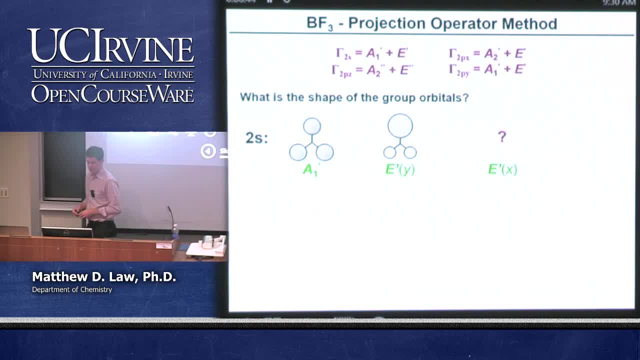 They are orthogonal And we'll get back to that point in a second. So we can use the projection operator to determine the E prime Y, But I mentioned that we can't use it to look at the E prime X. So the projection operator method in this way, the way that we're using it now, 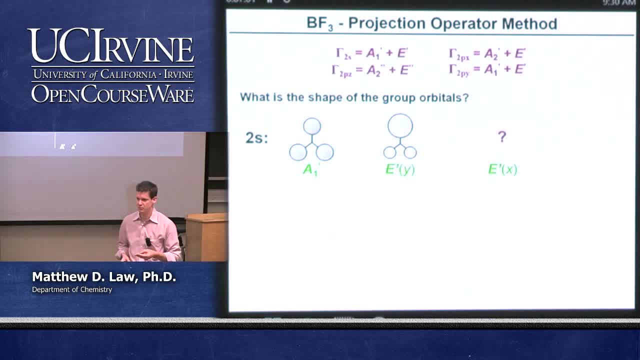 can only determine one of the two wave functions that's buried in the E prime And we have to use a different approach. We're going to use orthogonality to determine what that E prime X must be. Yeah question, So we know that is the EY, specifically because if we look at the Y axis, 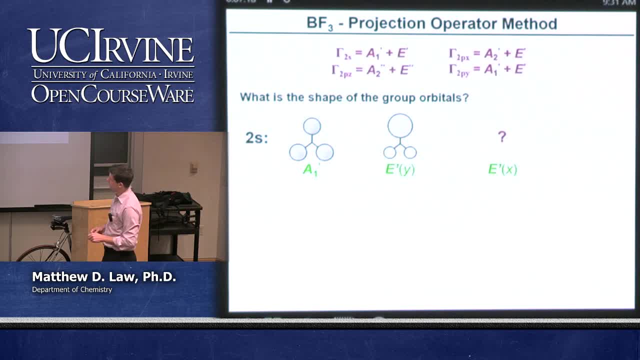 it would be perfectly, I guess, positive opposite. Yeah, so the way that this has Y-like character is because the wave function is negative down here and positive up here. Okay, That passes right here, where it changes from negative to positive. 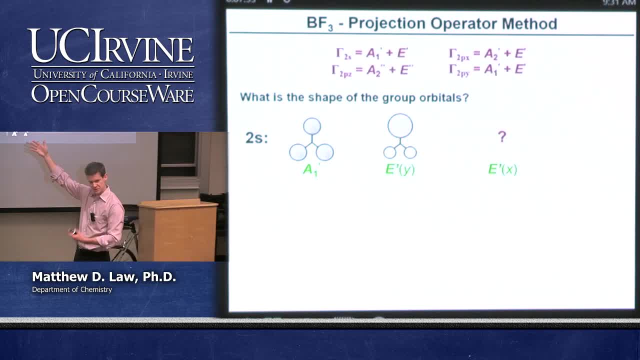 And so that's just like the Y axis: It's positive on the upper part, It's negative on the lower part And there's a node, if you will, that's right through this plane. That's the way, it's the same. 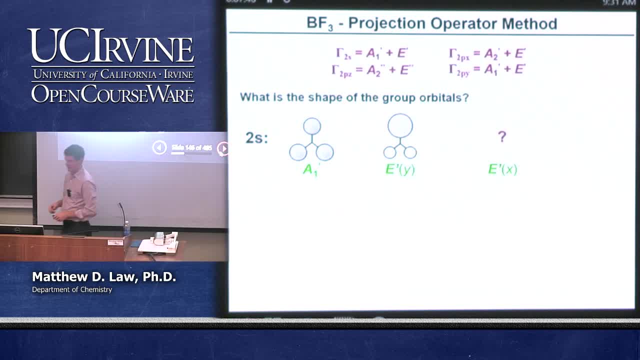 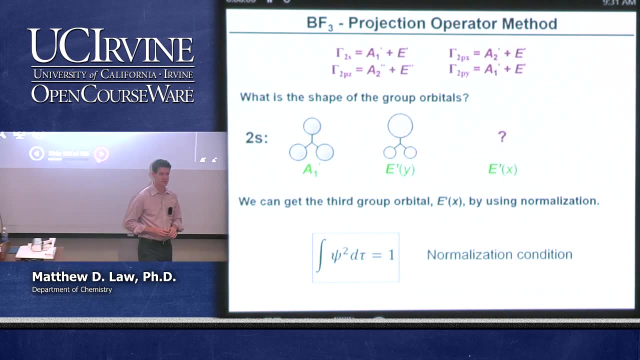 Okay, So let's look at generating E, prime, X, now the final one. So we can get this third one by using normalization and orthogonality. So let's determine how we can do that. Remember from the beginning of our discussions of molecular orbital theory what normalization is. 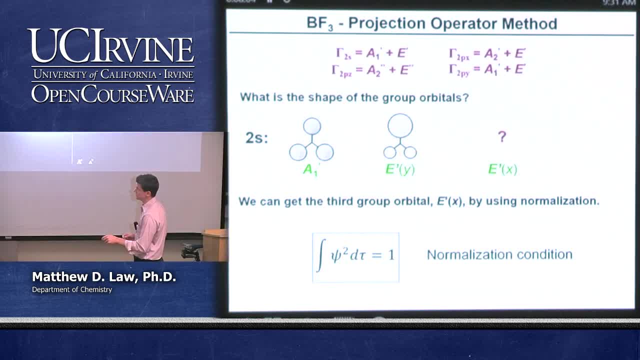 It tells us that when we take the square of the wave function- this is the molecular orbital wave function- and integrate over all space, the probability of finding an electron there must be equal to one. Okay, So when the wave function is properly normalized, we have the overlap integral over all space equaling one. 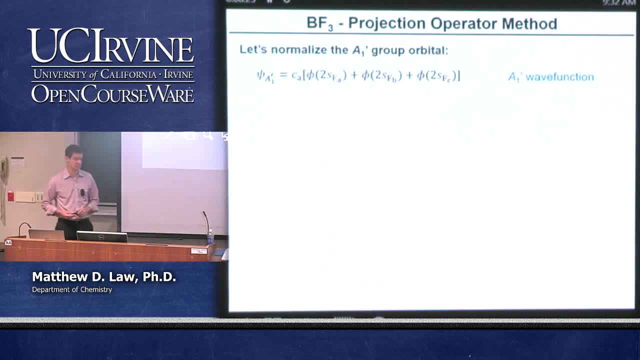 Okay, So let's normalize these wave functions that we have. Okay, We're going to normalize the two that we've got and we're going to use that result then to determine what the third one must be. Okay, So the first wave function is the A1 prime. 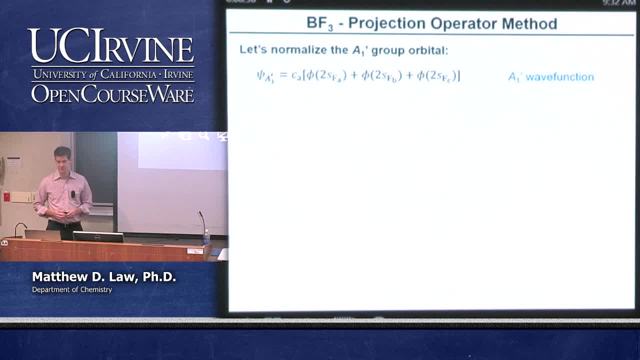 Okay, Which we said was an equal mixture of the three different 2s orbitals, Right, All positively signed, And so this is the problem that we want to solve here: We want to determine what this coefficient must be in order to make this wave function normalized. 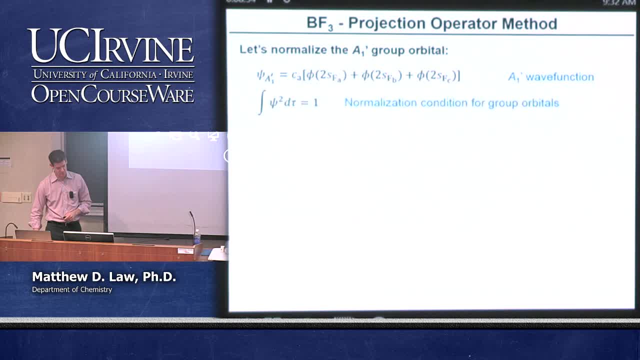 Okay, So that's the wave function itself To determine the normalization we want to determine, and set that integral equal to one. Okay, So let's do the integral, And this is the integral of the function squared Right. So this is what this is telling us. 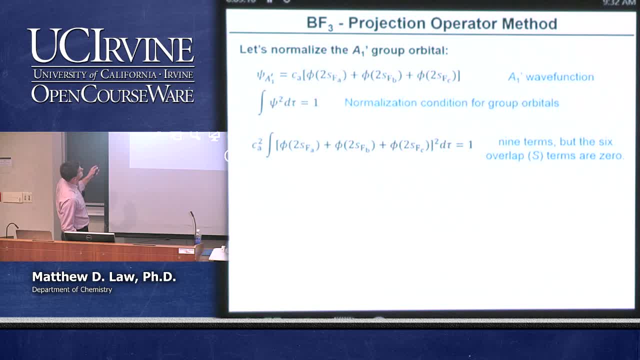 We need to take the function squared and integrate over all space. The CA. right, the coefficient comes out front because it's just a number And what we're left with is a series of integrals. Right, A sum of integrals. 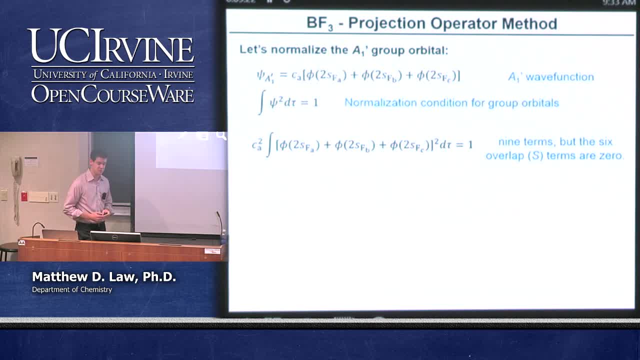 And it turns out, if you do the multiplication, there are nine integrals that you would need to do in principle, But only three of those are not zero. Right, Because the orbitals that are in the group orbitals are so far away from each other that there's no overlap between the three that are, you know, the three fluorines. 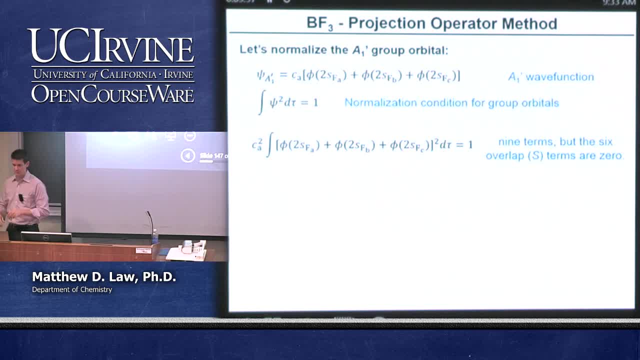 The only products that are non-zero are the overlap of the orbitals with themselves. Okay, So we have these three terms as the only ones that are not zero, Right Where we have the square of the orbital on FA, the square of the orbital on FB, the square of the orbital on FC. 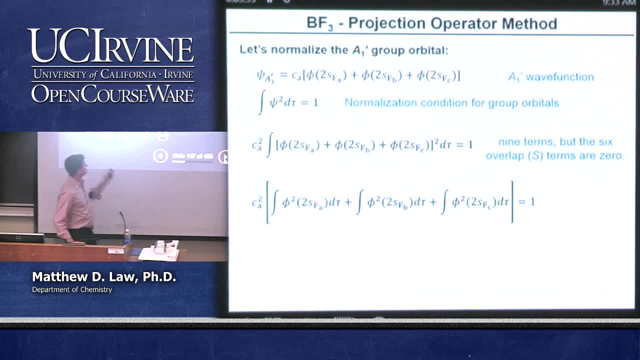 Okay, And we know that each of those integrals is equal to one because the atomic orbitals are individually normalized. Okay, Remember that the atomic orbitals come in normalized. The molecular orbitals are not necessarily normalized. until we do it, Okay. 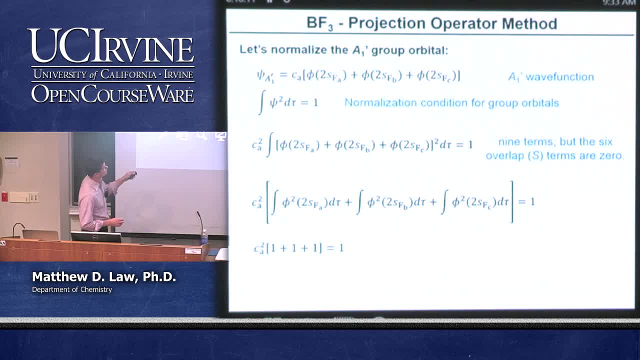 And so what you have then? these three, the only three integrals that are not zero are both are all equal to one, And so you have CA squared multiplied by one plus one plus one equals the normalization condition of one. So in other words, three times CA squared is equal to one. 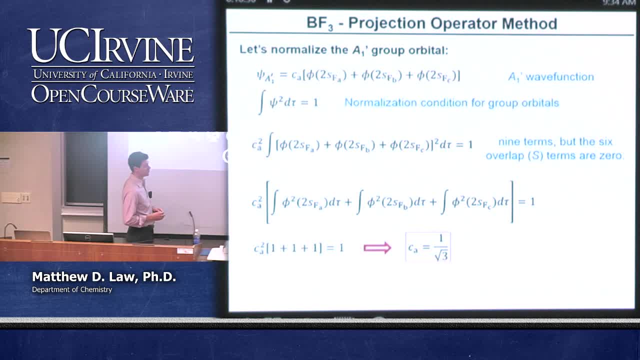 We can solve then for what CA must be. And CA is equal to one over root three. Okay, And so that is the coefficient that goes in the original molecular orbital wave function in order to make the molecular orbital wave function normalized. Okay, So the coefficient for each FA, FB and FC are the same, as they must be. 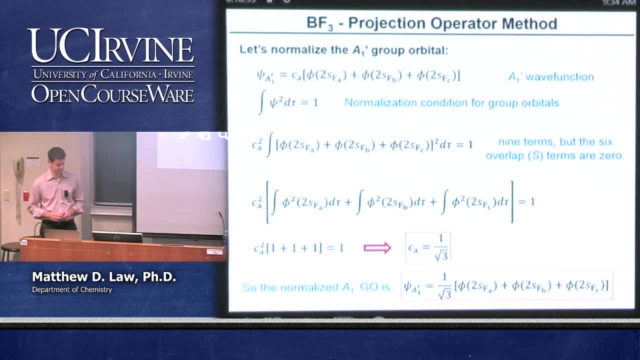 Okay, So we have a finished molecular orbital wave function here. So we can do that for the first one And we can also do that for the second one, the E prime Y. Okay, So let's look at the E prime Y next. 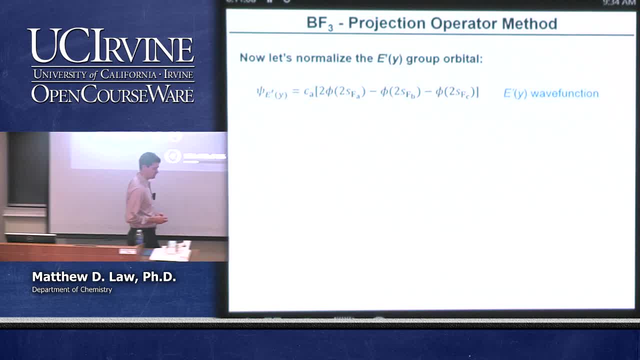 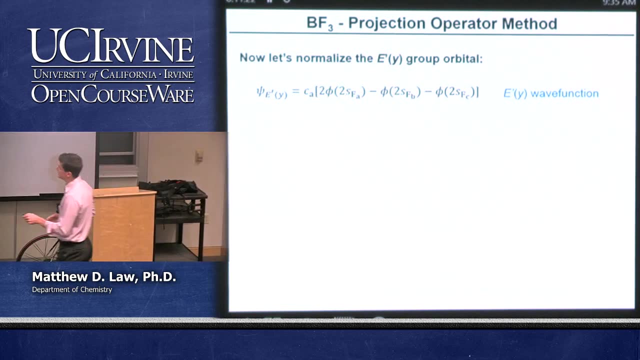 So here's the E prime Y problem. Remember that the wave function here has twice the amount of FA character and negative signs for both FB and FC. All right, So this is twice the amount of wave function from FA Minus FB, Minus FC. 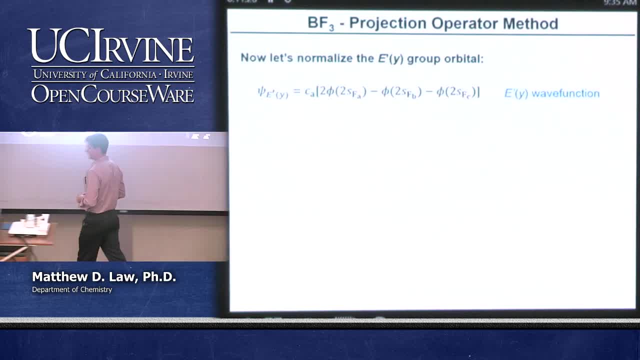 And we want to determine what the coefficient is. that's sitting out front there Again. the way that we do that is by requiring the function to be normalized Again. the only integrals that are not zero are those with the individual atomic orbitals and themselves. 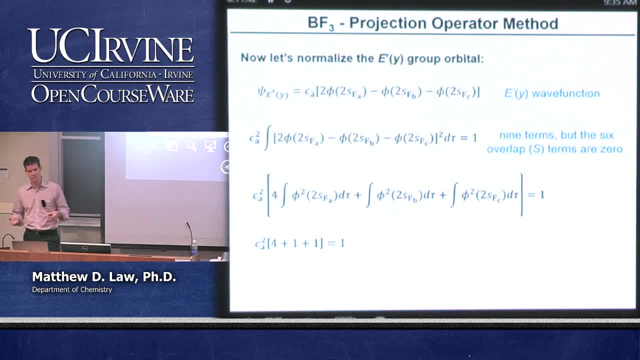 Okay, And so you again have a product, a sum of three terms, Each of the terms being equal to one. Okay, So each of these integrals is equal to one. Remember, we square it So that squares two to four, And we can pull four out front of the integral, because it's you know, it has no functional form. 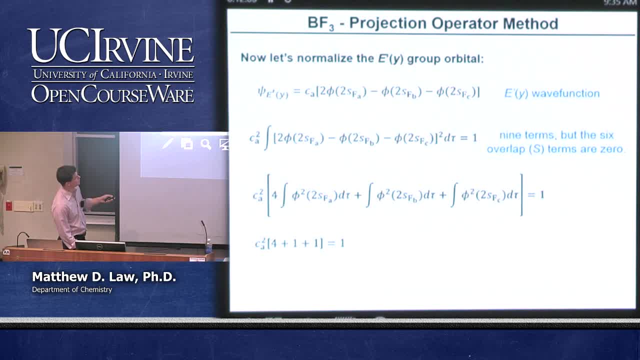 And what we're left with is four plus one plus one, That's this here equaling one. Okay, And so we can solve then, for what CA is, And CA in this case is going to be one over root six, And that would give us our normalized wave function for the second molecular orbital. 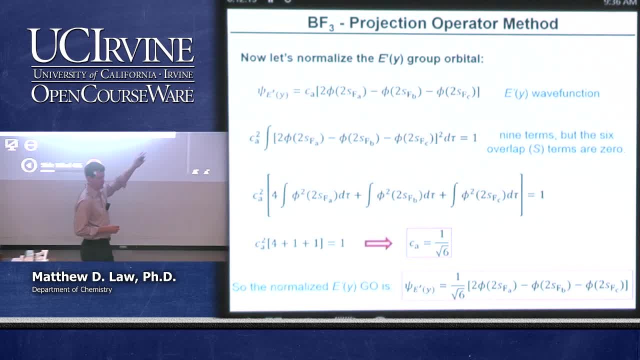 One over root six, Twice FA Minus FB, minus FC. Okay, That makes those wave functions properly normalized. We can take this information, this normalized, these normalized wave functions and in particular this coefficient from the first two to determine what the third molecular orbital must be. 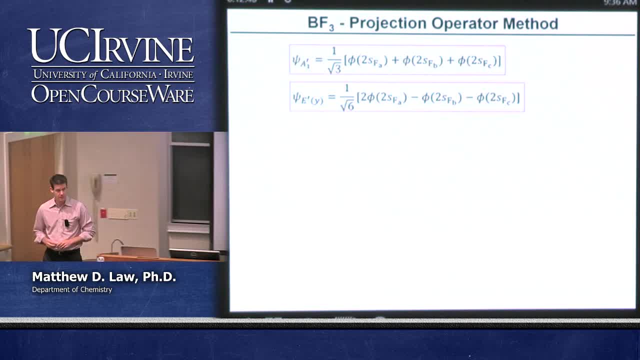 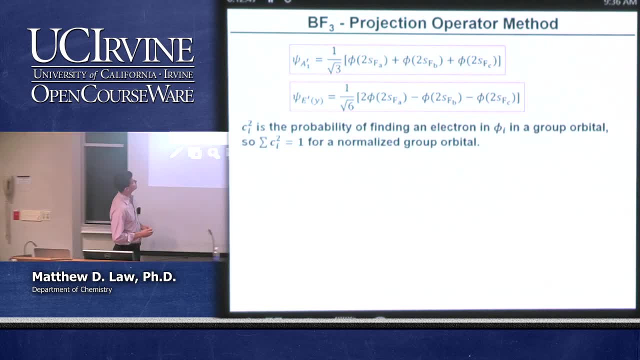 Okay, So here are those first two wave functions. The question is, what is the third wave function? Let's see how that we can figure this out. Okay, So I can't see the screen sometimes here. So one of the things to remember is that the coefficient squared, as we've talked about before, gives us a probability. 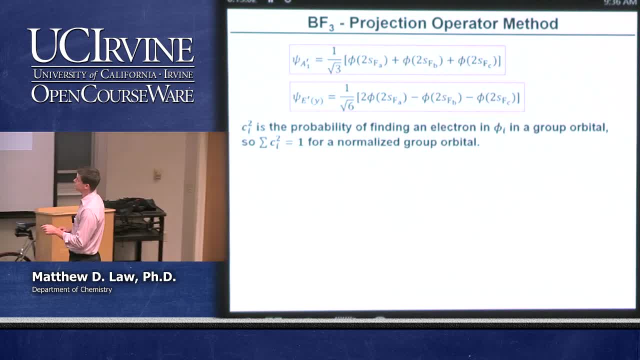 All right. It gives us a probability of finding the electron in a particular atomic orbital within the group orbital, And so one important thing is that the sum of the squares of the coefficients is equal to one for a normalized group orbital. So, for example, each of these has equal contributions of one over root three. 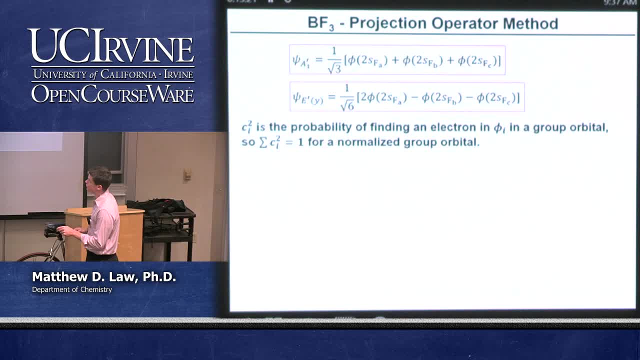 If we square one over root three, we have one third, And if we add one third for each of the orbitals we have one. So we have equal probabilities of finding the electrons in each of those equivalent orbitals And we have a probability of finding electrons somewhere in that molecular orbital of one. 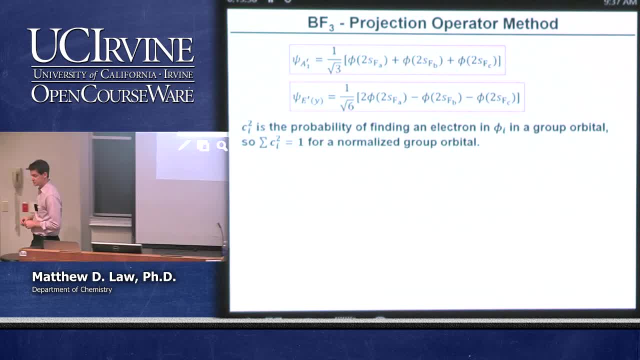 And it's the same thing for the second one. Okay, In the second case, if we square the coefficient right, what we're going to have is two divided by root, six squared. That gives us two thirds. Okay, And this is going to be one sixth. 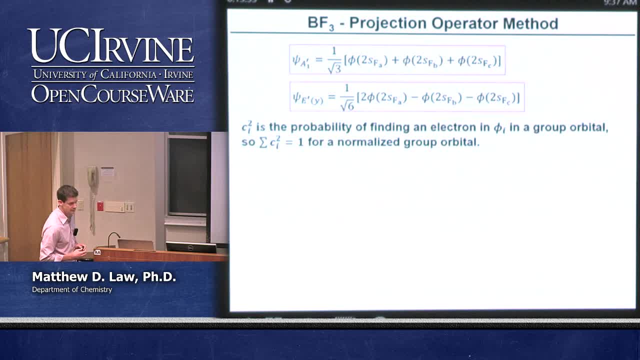 And that's going to be one sixth when we square the coefficients, And so two thirds plus one sixth plus one sixth gives us an overall probability of finding the electron of one. So that's how that normalization works out. We can put this in a table. 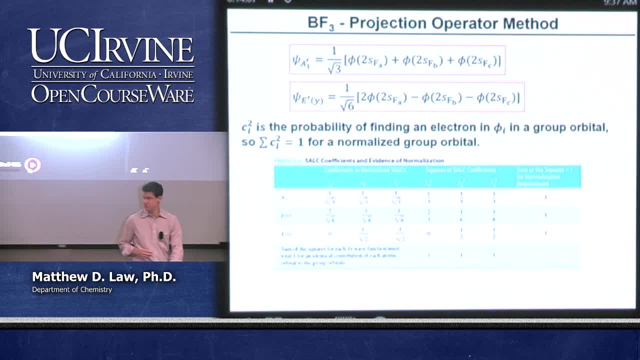 This is a table that's taken out of your book to show exactly how these coefficients look. So here's the molecular orbital wave function for A And here's E for the Y, And what we want to find is E for the X. Okay, 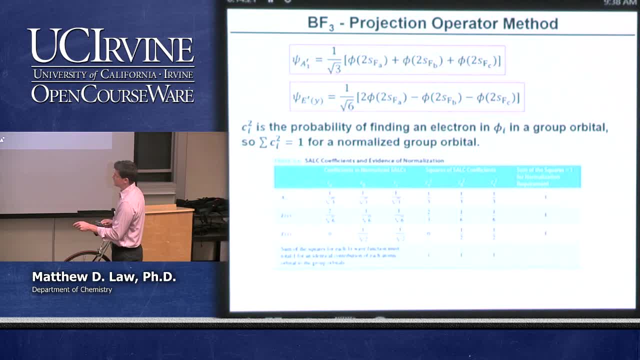 So ignore this line for a second. What we have for A is one over root three for each. What we have for EY is two over root six, negative one over root six and negative one over root six for the A, B and C atoms. 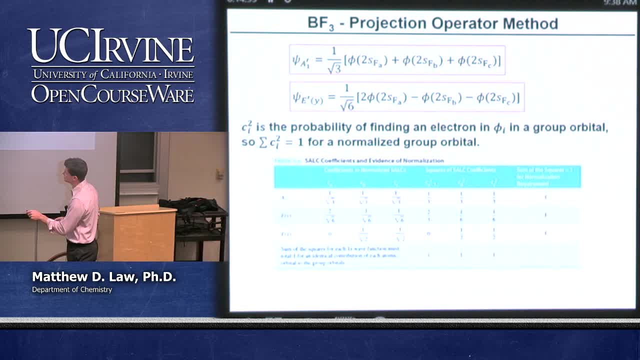 Okay, If we square the coefficients- these are the coefficients here- If we square them here, we get one third, one third and one third. And if we square these to get the probabilities, we get two thirds, one sixth and one sixth. 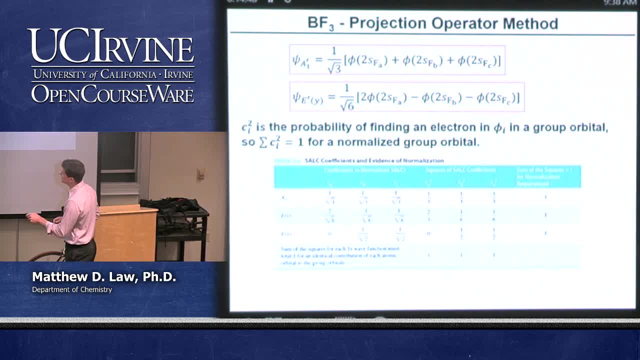 Okay, And of course the negative drops out. You sum these up and you have a probability of one. You sum these up and you have a probability of one. Okay, The third wave function must be the same kind of deal. Okay, We must have a set of coefficients that when we take the sum of the squares of their coefficients, we get a probability of one. 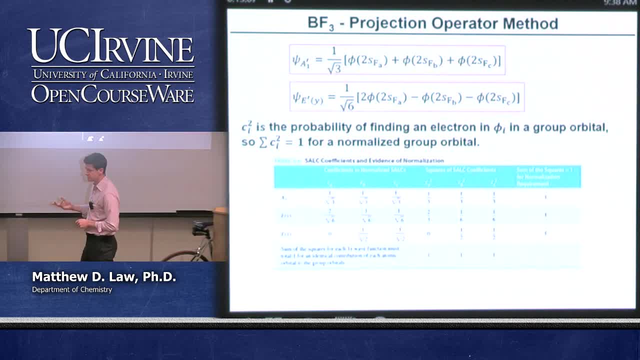 The other thing that must be true about this third wave function is that when we consider the contribution of each of the individual atomic orbitals to the overall set of molecular orbitals, all three, each of the contributions from A, B and C considered all together, must be equivalent. 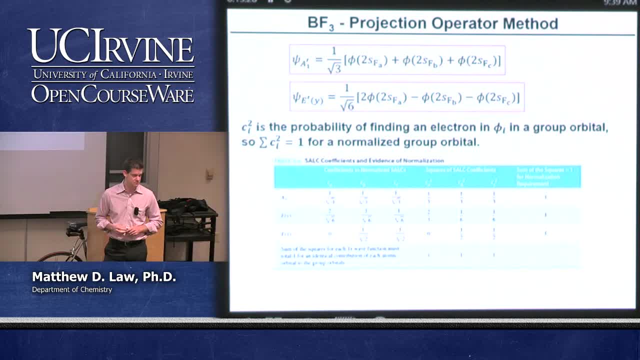 And that's because the orbitals themselves are exactly the same Right, And so, for example, the amount of character coming in from A1, from atom one, must be equal to one, The second one must be equal to one, And the one coming in from the third atom must also be equal to one. 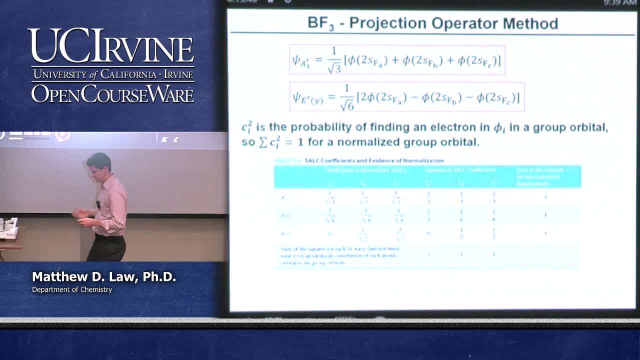 Okay, This is because the orbitals are equivalent. Okay, So we can't have one of the S orbitals contributing overall more electron density to the full set of molecular orbitals. It's just symmetry forbidden. So how are we going to organize that? 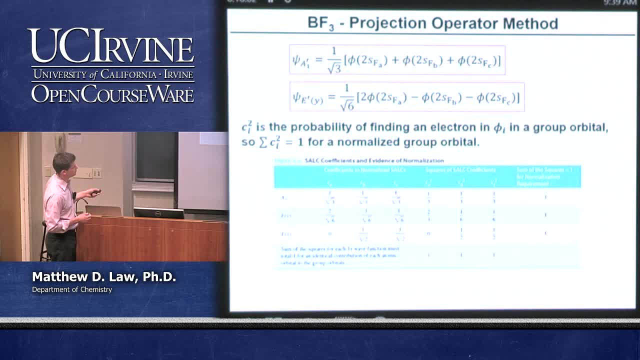 Well, if you look here at the first atom, atom A, and sum up the probabilities, the coefficients squared from A1 and EY, we already have one together here, Right, Because EY comes in with twice this big fat lobe on atom A. 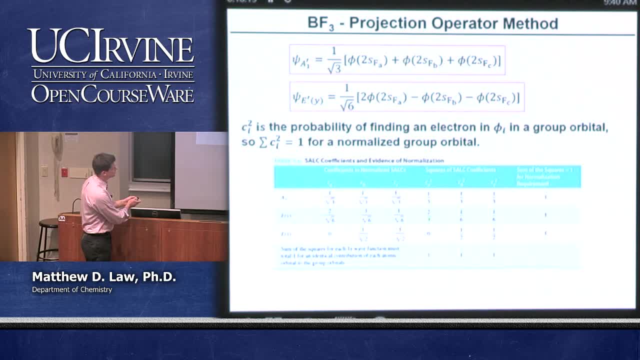 Okay, And so we already have one-third plus two-thirds, So we already have a full contribution from atom A. That must mean that the contribution coming in on atom A in the EX orbital is equal to zero. In other words, there's no contribution from atom A. 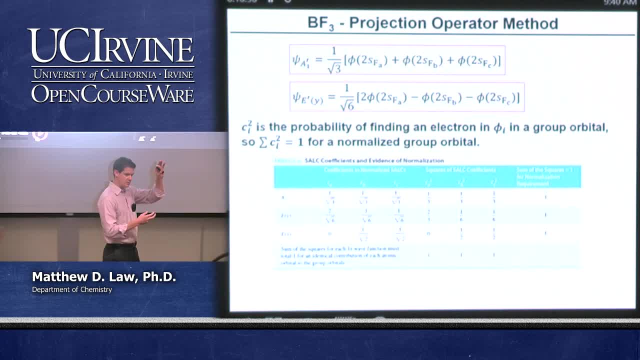 Okay, If there's no contribution from atom A, then the contributions must come from atom B and atom C only. Okay, And the only way that we can do that and again satisfy these sum rules is that the contributions must be the same from atom A and from atom B and from atom C. 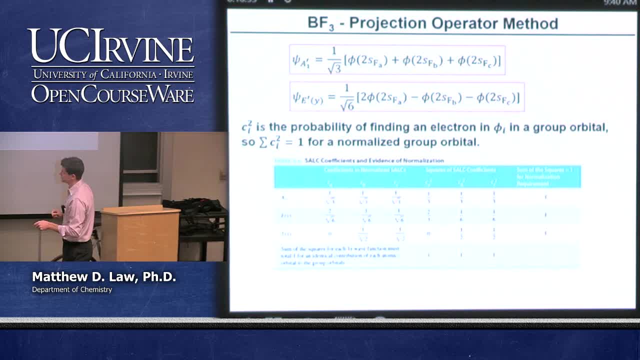 And in this case, in order to make sure that it's got X-like character, we have to have the difference between them. One of them has to be negatively signed, Otherwise there's no way to build a molecular orbital that has the symmetry of the X axis. 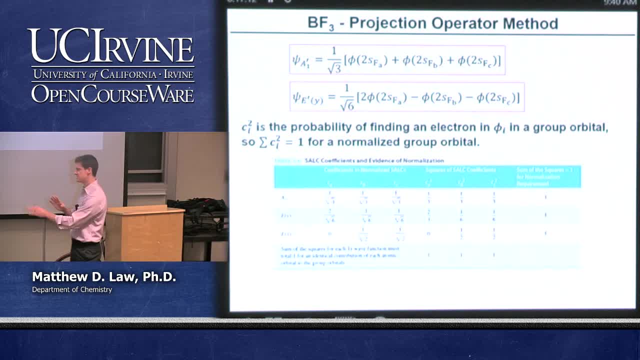 Okay, So we have to have going along the X, we have to go from a positive to a negative situation with a node in between. Okay, So if we have no character from atom A and we only have character from B and C, then the coefficients necessarily must be one over root two. 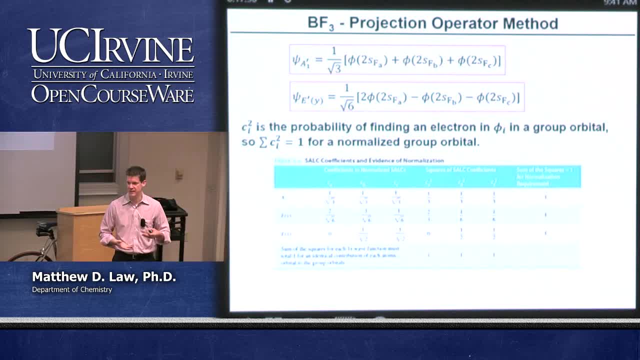 Okay, Because one over root, two squared is one-half. One-half plus one-half is equal to one, Okay. And we have a negative sign, in this case just on the C atom. So our molecular orbital is going to be negative, Okay. 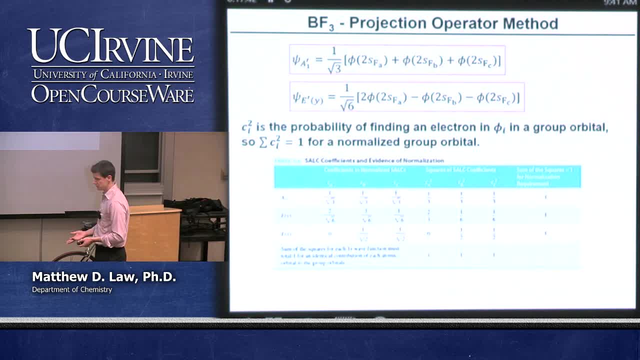 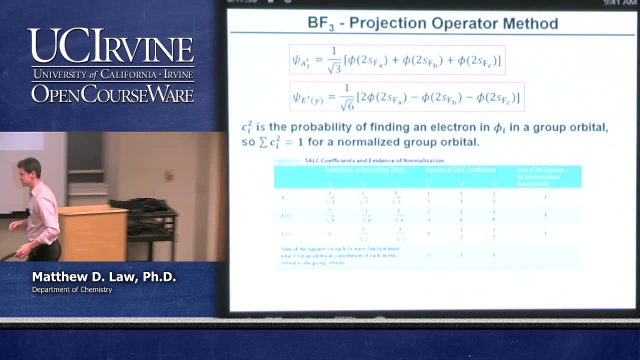 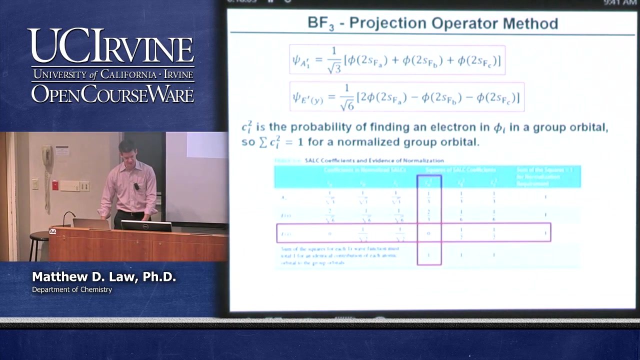 So our molecular orbital is going to be one over root, two orbital B minus orbital C, And then that will give us equal contributions from each individual atomic orbital and normalized individual molecular orbitals. I forgot that this doesn't work. Okay, And so that's what this highlighting describes here. 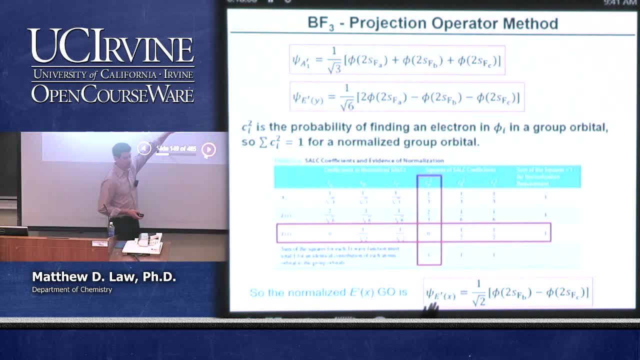 So the take-home here is that the orbital that we're looking for, Okay, must have this kind of wave function: No contribution from atom A equal, but opposite contributions from B and C. And so let's look and see what this must look like. 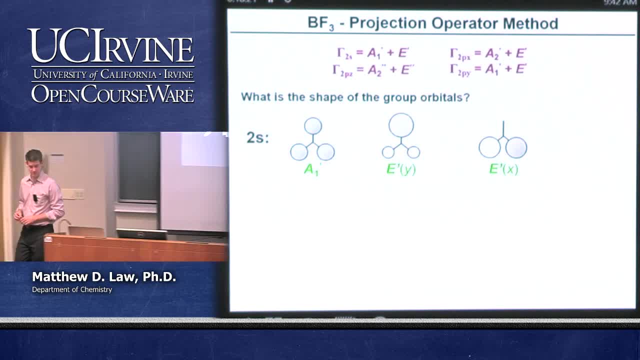 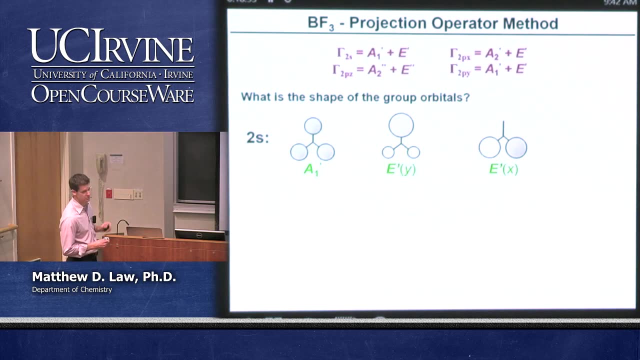 We paint that in, It's got to look like this, Okay, So there's no contribution from A, There's equal and opposite contributions from B and C, And the coefficients are one over root two. So that means these orbitals here are a little bit bigger than the original, which were shared between three equally. 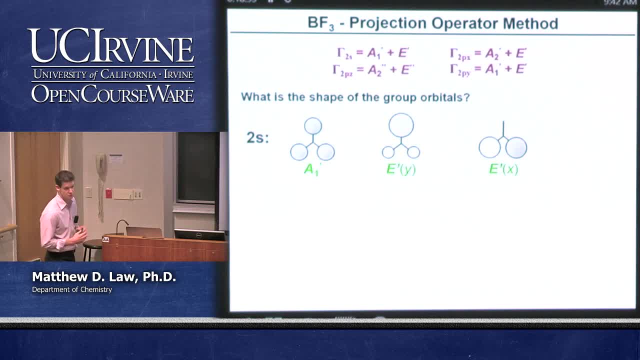 Okay, These are all one over root three. These are all one over root two. All right, So those orbitals are a little bit bigger, indicating that their contributions are larger. You can see that it has x-axis like symmetry, because this is the x-axis here. 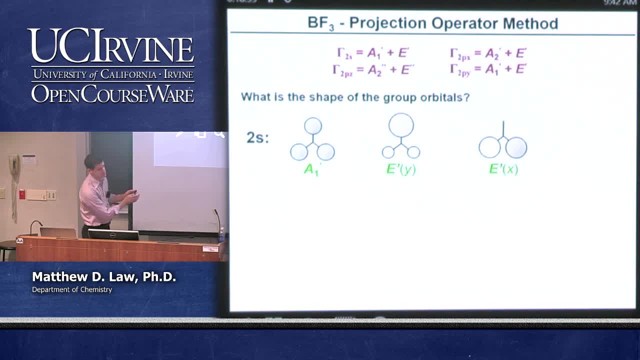 And we go from negative to positive and there's a node that runs between them, just like the x-axis would have. Okay, So this is the general idea. So we can use the projection operator method to always get all of the molecular orbitals that are just one by one. 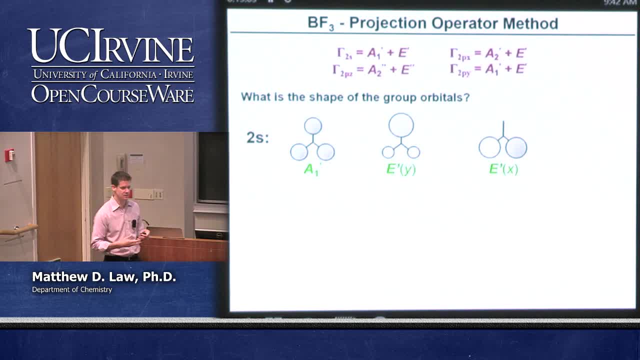 These are just one by one matrices, So any A or B we can automatically get from the projection operator method. Anything that's got a two by two or three by three, like an E or a T, we can get one or two out of them from the projection operator method. 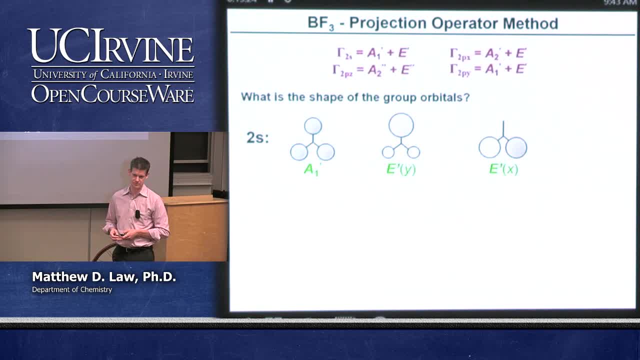 And then we can use orthogonality and normalization to get the last one to finalize our set of molecular orbitals. Question: How do we assign whether xB or xC is a negative sign? Yeah, In this case it does not matter. 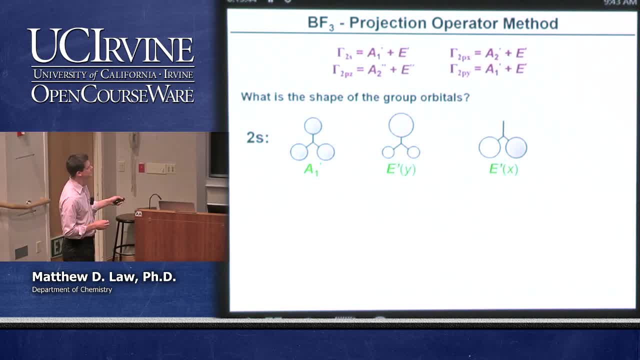 It doesn't matter. So if you look at making sure these are all mutually orthogonal, they would be mutually orthogonal even if the sign on this was flipped. Yeah, So yeah, it was just arbitrary. It has to be one or the other. 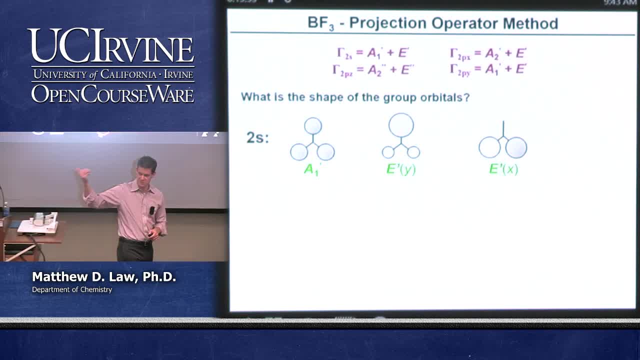 To keep the shading consistent, we chose the dark positive lobe to be on the positive side of the x-axis. But yeah, it doesn't really matter. Other questions about this one. Yeah, How do you know that one has to be positive and one has to be negative? 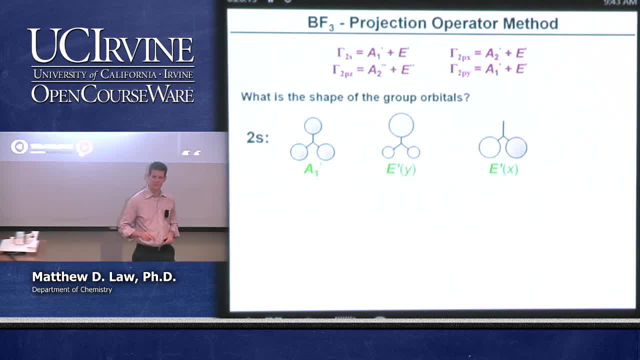 Okay, that's a good point. So how do you know that? There are two ways that I can point out that you can know that. One is that this orbital here has to have x-like character, And if both of these lobes were positive, there wouldn't be any node. 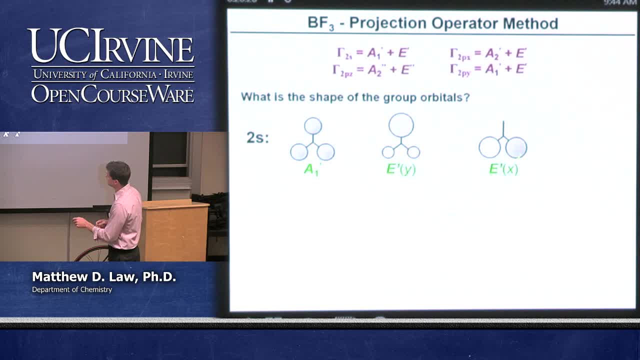 There wouldn't be any x-like character to it. The other thing that you can notice is that if both of these were positive, then this orbital here and this orbital here, for example, would not be orthogonal, So they have to be mutually orthogonal. 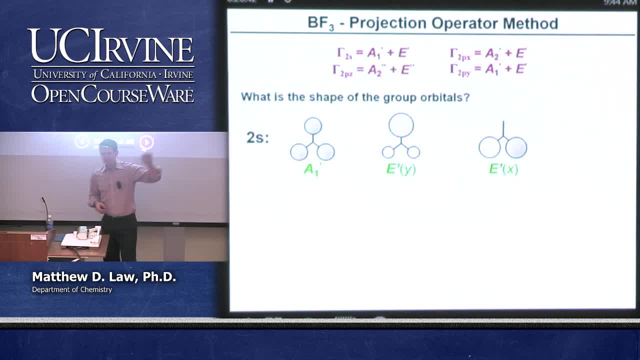 What that means in reality is that each of these orbitals- here the molecular orbitals- is independent of the others, So they don't have character of one in the others. They're all linearly independent functions, And if we didn't have the difference, if we took the sum, we wouldn't have that orthogonality. 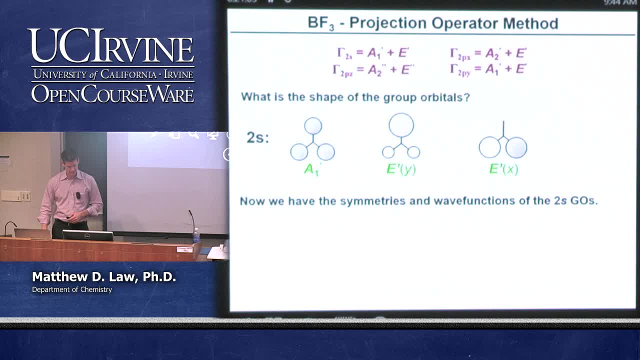 Okay, So let's see if we can move on here to finish up the molecular orbital diagram for boron trifluoride. Okay, So the idea is we did this for the two S's just because they're the easiest to see, But you could definitely do this for all the two P's. 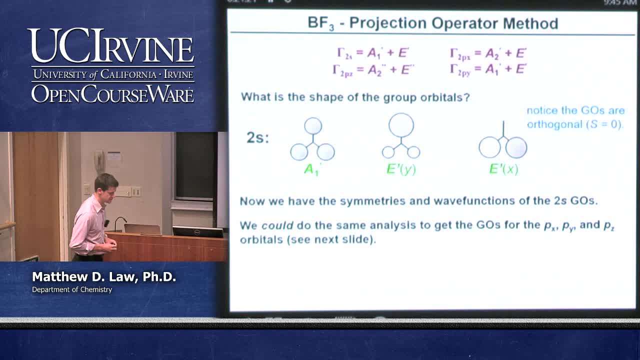 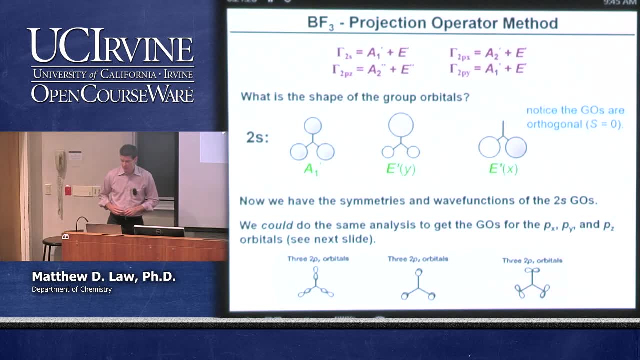 And the procedure and the results in fact are almost identical, So you'd get the same sort of look to the orbitals. We're not going to do the P's explicitly, I'm just going to show the results. But you could do the same thing with the P's. 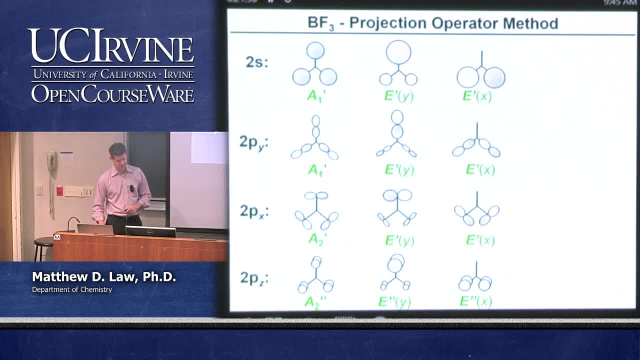 The PY's, the PZ's and the PX's, And this is what you're going to get. Okay, So these are the 12 group orbitals that you would get from the set of borons. These are the three from the S's that we just derived. 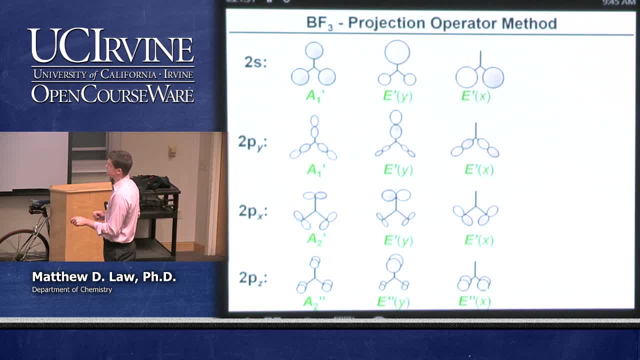 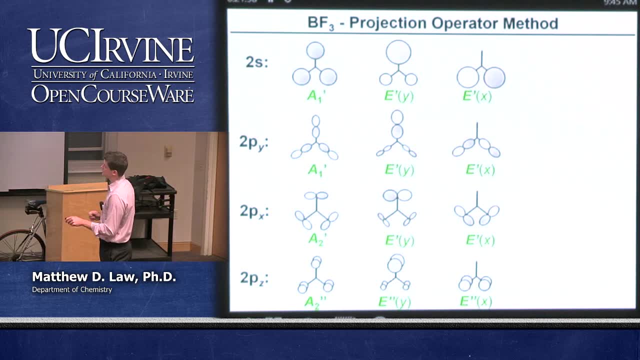 You can see. let's see, the two PZ's are exactly the same flavor. Okay, This one has a fatter lobe, This one has no lobe, But it's just an equal contribution of the two bottom ones And it's really the same for each set, the PX's and the PY's. 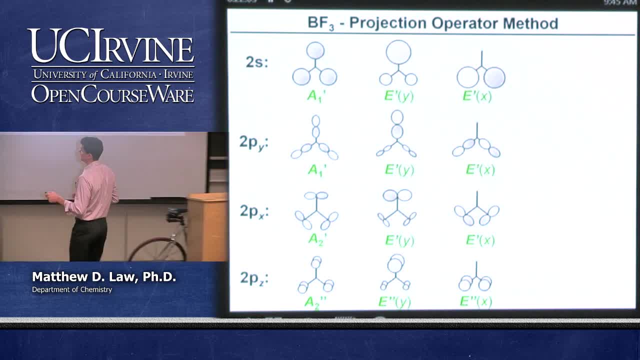 Drawing them is just a little bit trouble because you know you've got all these different lobes that you need to account for. But I hope you can see that essentially, that you get the same sort of flavor for each of the different kinds of orbitals. 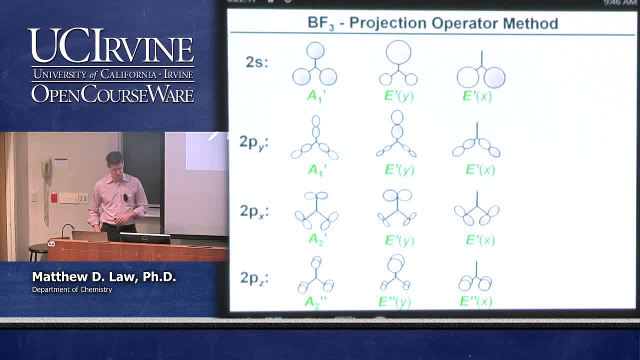 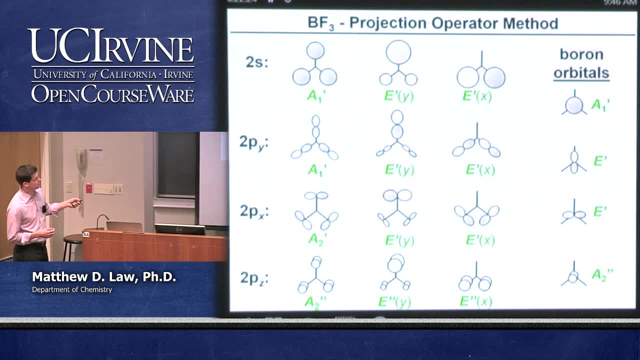 And this could be done rigorously by using the method that we just went through. Okay, We have the results of what the group orbitals look like and what their symmetries are. We want to look, then, at what the center atom orbitals symmetry is. 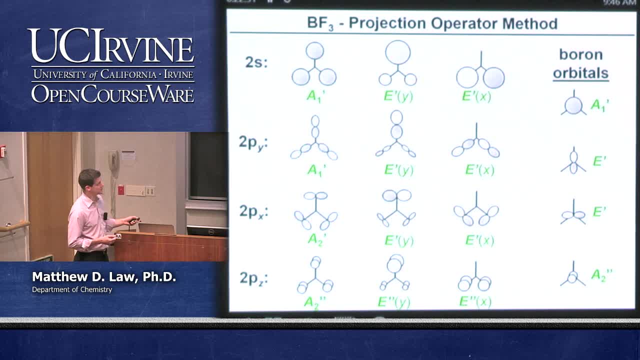 We can just read this right off the character table again: The S is totally symmetrical, The S is totally symmetric. And then we can determine what the PX, PY and PZ's are going to look like. And they have those symmetry labels. 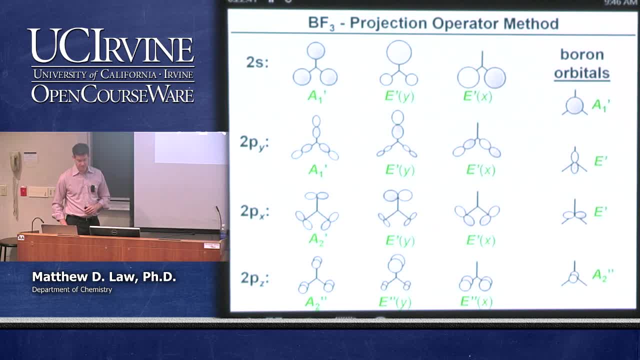 Then we just complete the diagram like we normally would. Right, We assign the interactions, So A1 has those interactions, The next one down Right, We have A2, prime Right, Which has one pair to deal with, And then the big set here are the Es. 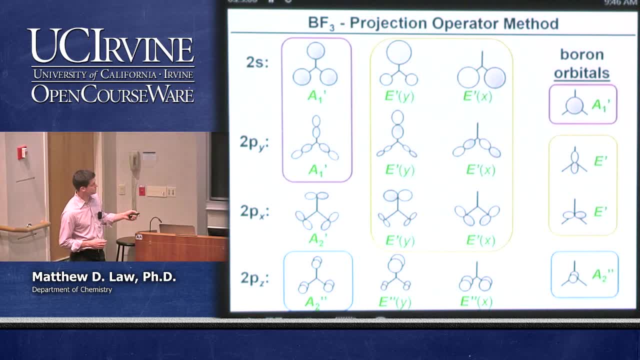 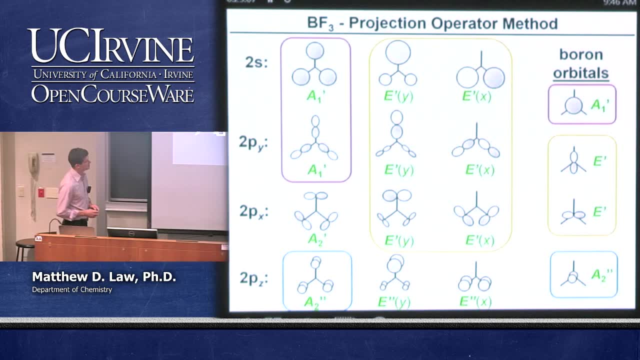 Right. So the Es from the center atom And the Y orbitals Have a significant number of possible interactions with the Esets on the group orbitals, And then the others are independent. So the A2 prime's got no partner. The E double prime doesn't have any partner on the center atom. 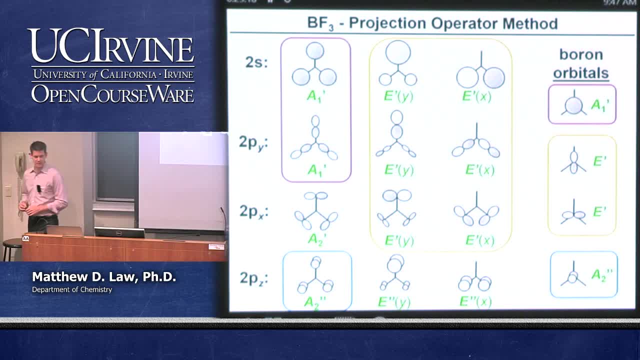 And so those are going to be non-bonding Okay When we build the molecular orbital diagram in a second. One thing to realize is that not all of these interactions with the E primes are of the same strength, And you can kind of understand that. 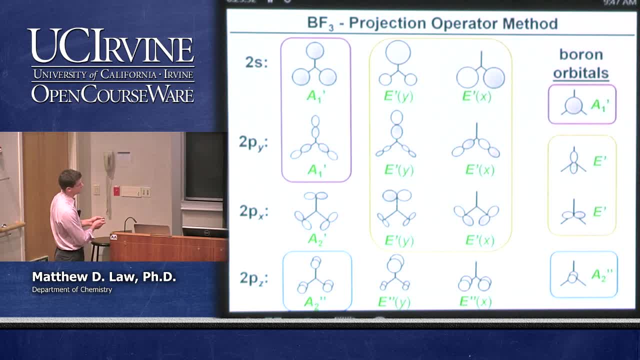 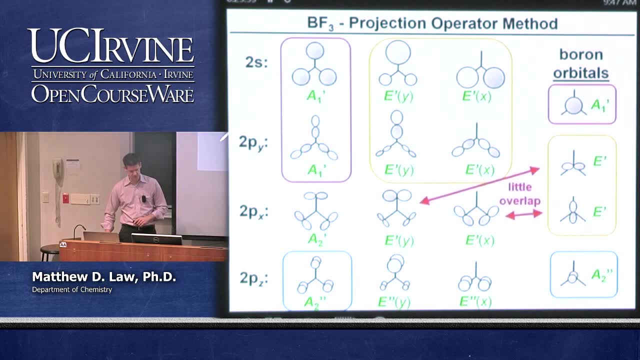 By just looking at how the center atom is going to interact with these different orbitals. Okay, And it turns out that one set of interactions here is going to be particularly weak And effectively non-bonding. Okay, So you can stare at these two interactions that I've shown. 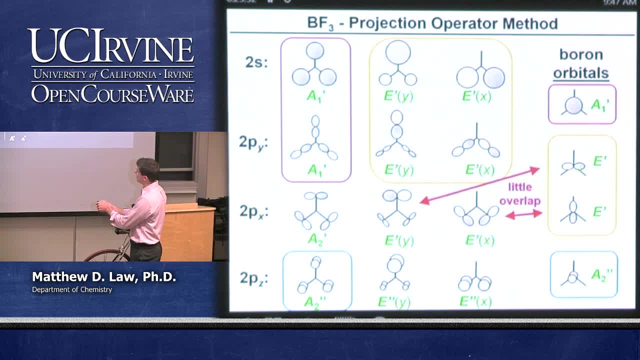 Right, This interaction between the X E prime from the center atom And this E prime, Right, This is Something is wrong here. But anyway, This center atom orbital interacting with this guy is not going to give us very strong interaction, Because we just have kind of a parallel interaction between this lobe and this lobe. 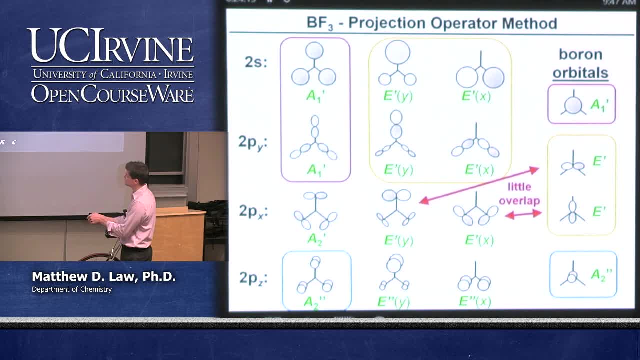 And these lobes are pointed away from the center atom And so we're not going to have very strong overlap. And this one and this one also are not going to have very strong overlap Because one of the lobes is pointed well away from the other two group atoms. 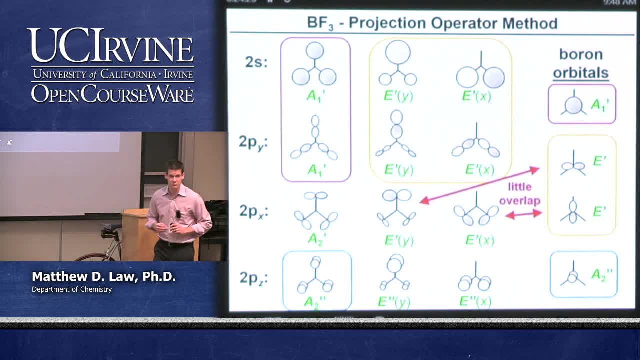 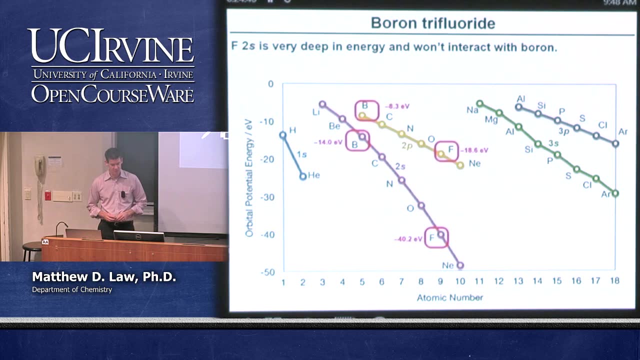 And the other one is kind of pointed between, And so we don't have very strong overlap at all. These two interactions are going to be mostly non-bonding in character, So let's look at the energy interactions that we have to worry about. 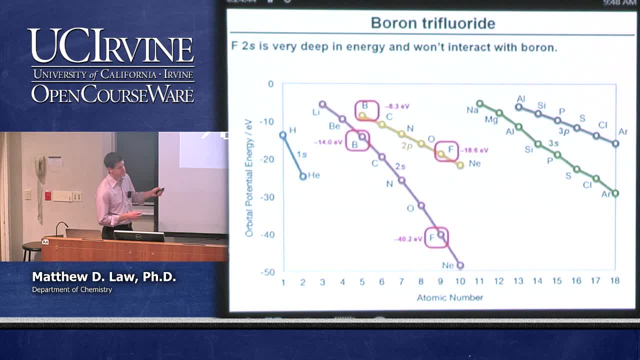 Boron trifluoride. The main thing to understand here is the fluorine 2s's are very deep and are going to be non-bonding. The other orbitals are all going to interact pretty well, And so here is our diagram. 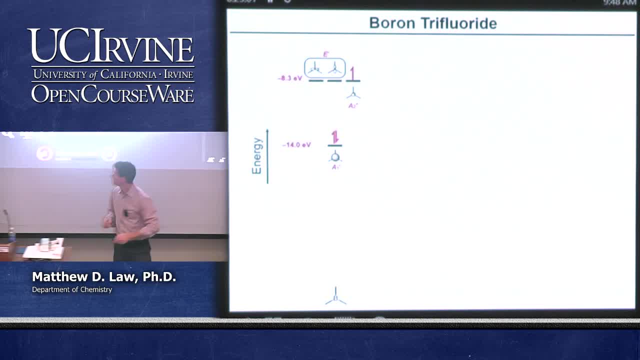 We have the center atom. here on the left We have our s and our p orbitals from the boron, Indicated with their symmetry A1' A2' and here's the E' set And their relative energies. We have 4 because we have a single boron. 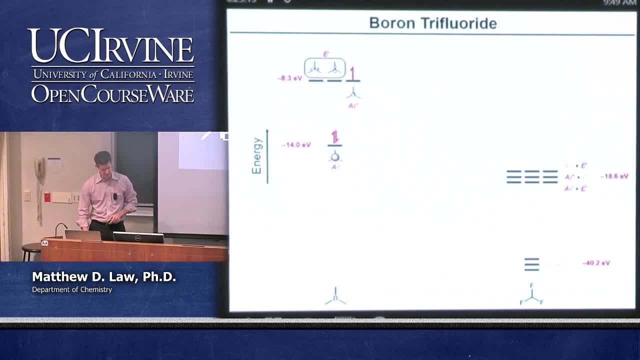 And then the fluorine group orbitals. coming in from the other side of the diagram, There are 12,. right There are 3 s's, There are 9 p's. Originally, they are all of the same energy And I've indicated their symmetry here. 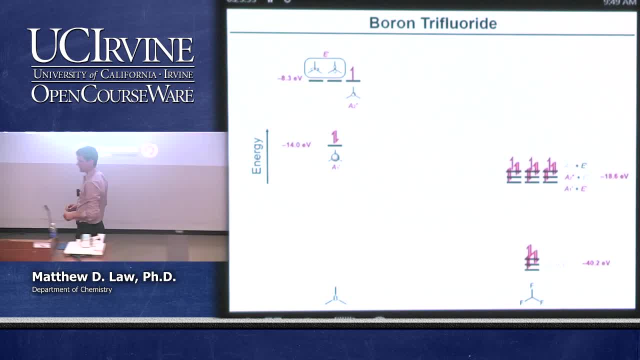 In these symmetry labels. Now we do our interactions. We start always with the sigma interactions. We can start lowest, That's easiest. The fluorines are so deep in energy that they don't interact with the borons- hardly at all- And so the 2s's just come across and they are going to be non-bonding. 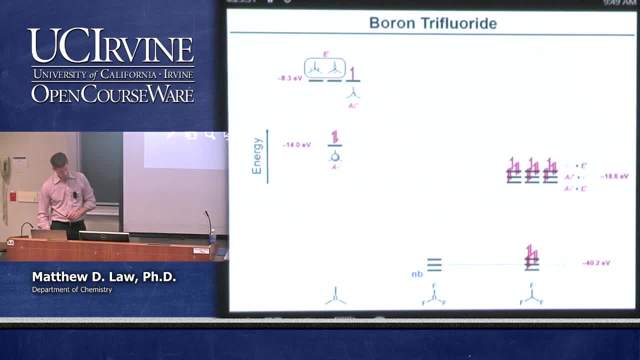 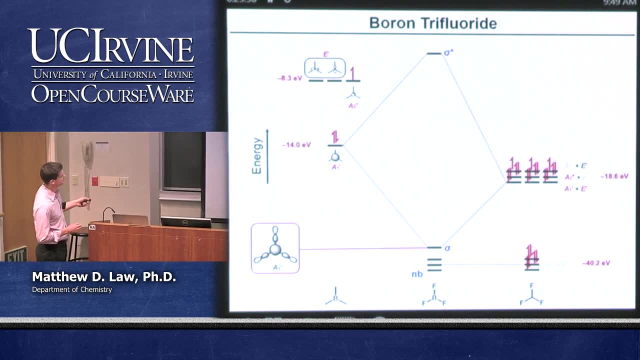 Almost completely non-bonding. And then we have some sigma interactions. Okay, We have the A1 set that we can continue to look at. The A1 is the s and one of the p's coming in. We make a bonding and anti-bonding combination. 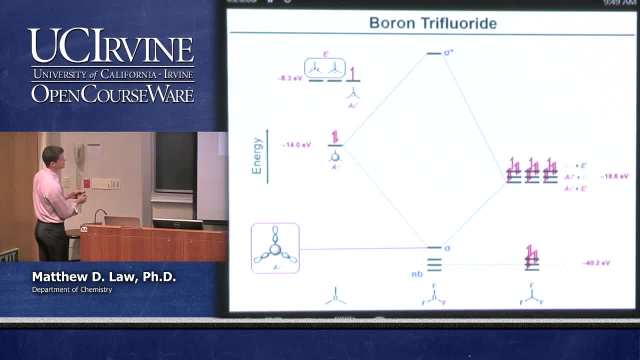 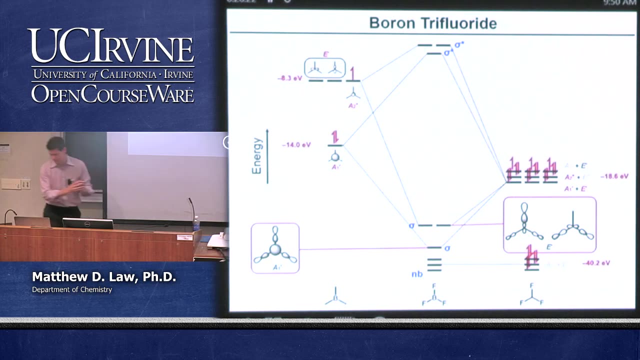 This is what the molecular orbital is going to look like, With the s mixing with the A1', which is the totally equivalent or totally symmetric molecular orbital, coming in. The other sigma-like interaction is this A2'. Sorry, we have the E's coming in first.